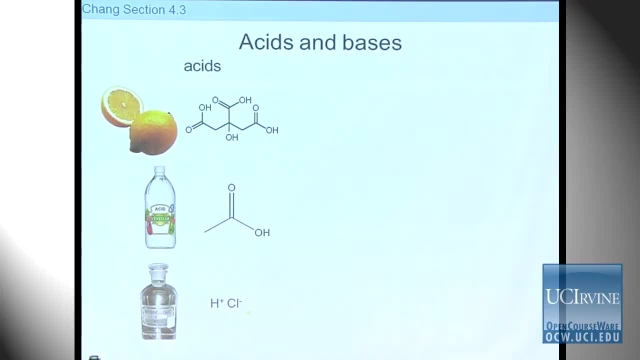 Of course it's an acid, because this H is fully dissociated from the Cl and hence you have H+ in solution, and that is the definition of an acid. On the other side we have bases: Ammonia, we've seen already, that's a base. 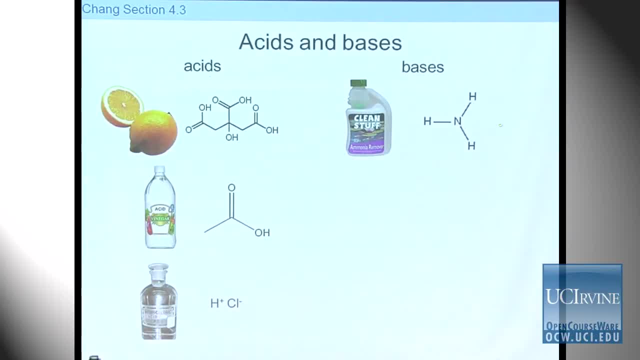 Why is that a base? Because the connections accept an H+. Okay, And so one definition of an base is that it can accept protons. Okay, And so one definition of an base is that it can accept protons. We'll see that spelled out in the next slide. 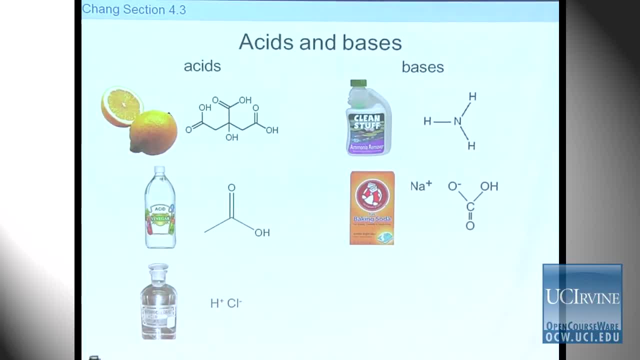 Here's another one. this is baking soda. It's also a base. Okay, so this ion here can accept another H+ And that's why it's basic. And then, finally, this is NaOH- sodium, hydroxide of caustic soda. 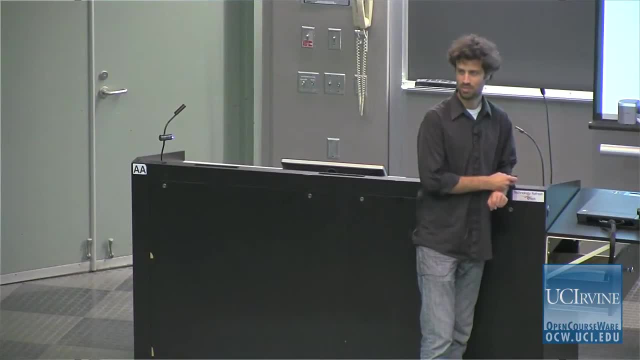 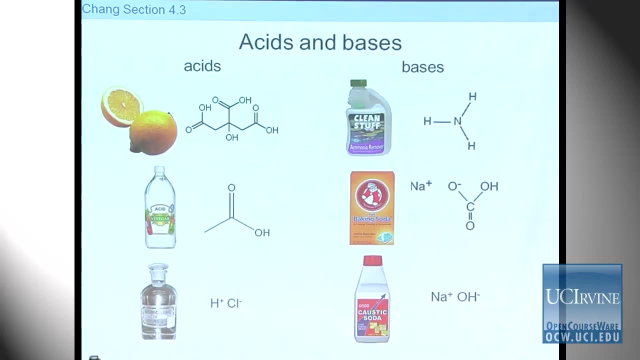 And this OH is highly basic. It is very happy to accept an H+, to accept an H plus in solution. So these are very common materials. you know you may have one of these things in your kitchen early. and so relevant chemicals and we have to understand how they're reacting, why they're reacting and what qualities they have. 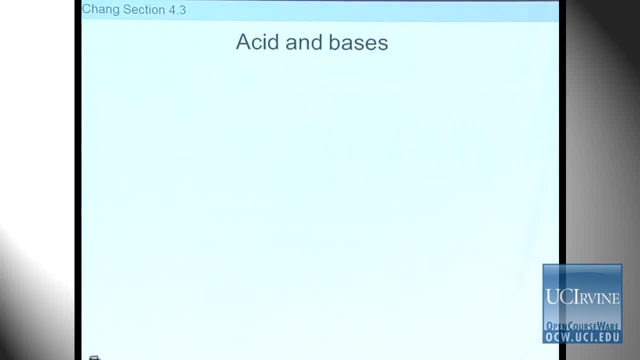 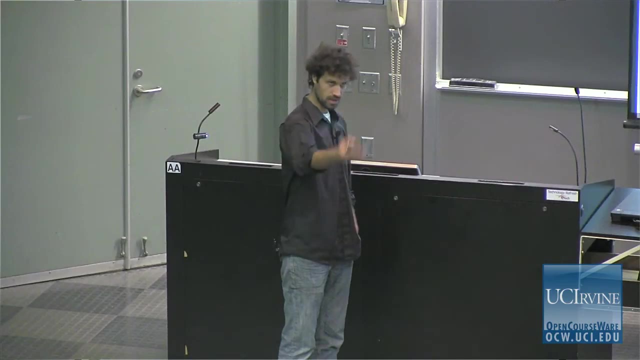 Okay. so let's look a little closer and come to a certain definition that we can use in this course. An acid we can define as a proton donor, Meaning that this H here that guy can split off from the compound and can be freely floating in solution. 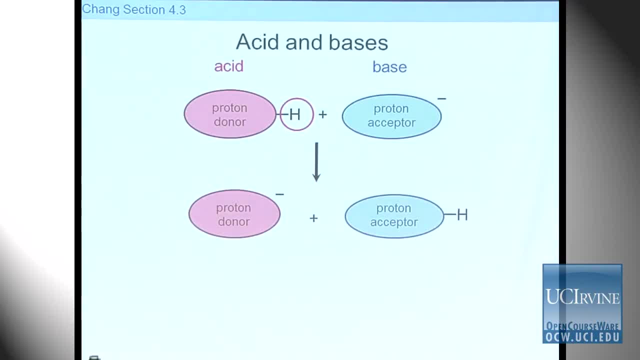 The base, on the other hand, can accept such protons. So there it is. So, effectively, what you have is kind of an acid-base reaction. You have an acid that gives off an H plus and a base that accepts that H plus and binds it. 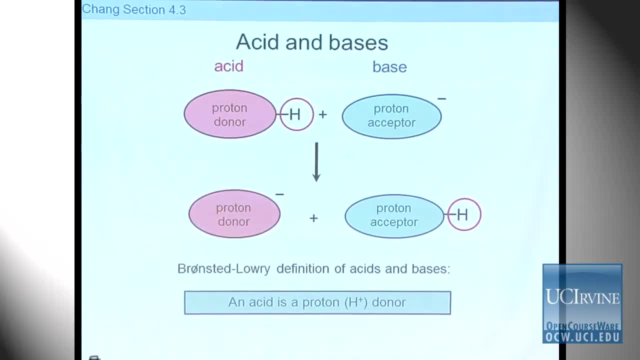 So this is one definition of a proton donor. There's more than an acid and a base. there's more definitions, but for this particular course, Chem 1P will use this definition: the Bernstadt-Lowry definition of acids and bases. 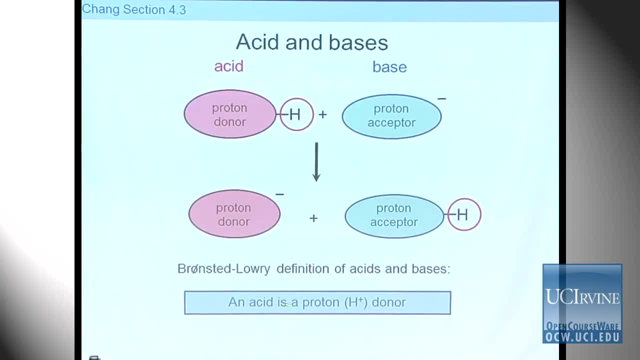 The definition is really what the graph is all about. An acid is a proton donor and a base is a proton acceptor. Very useful definition, But you'll see in Chemistry 1C there's more definitions of what an acid or a base can be. 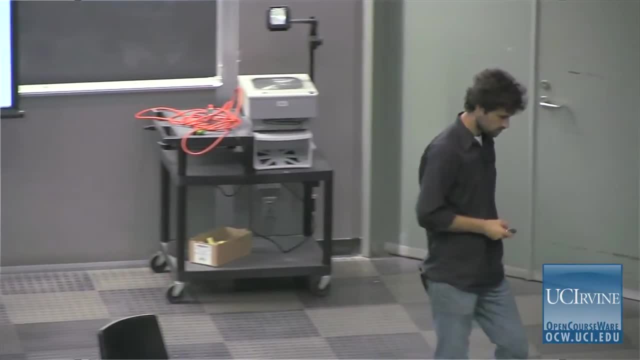 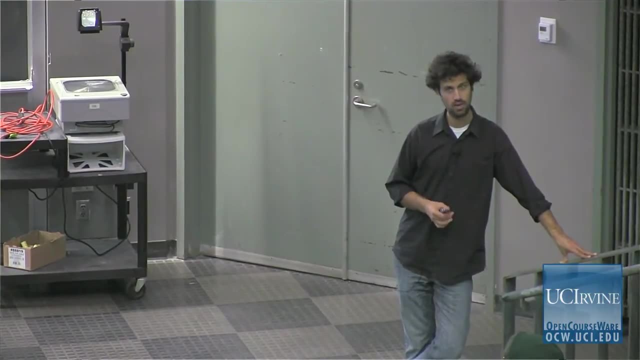 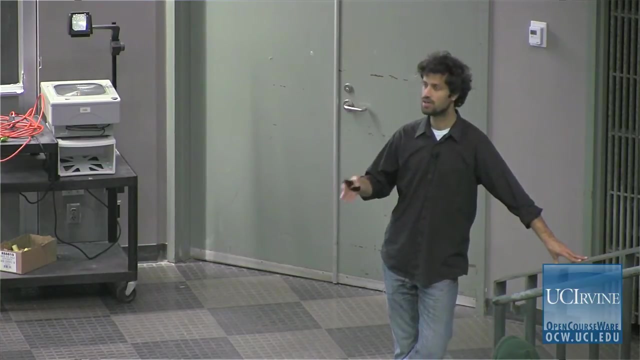 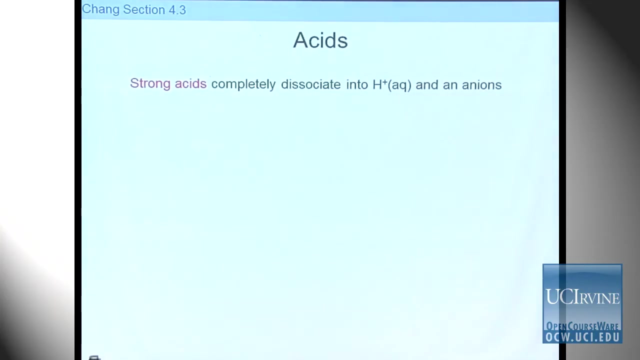 Okay Now, if you remember, we've seen several types of acids and bases already, And when we talked about strong and weak electrolytes, we saw that some of them are strong, other ones are weak acids, more strong and weak bases. So let me summarize that once again, because it's going to be important for this discussion. 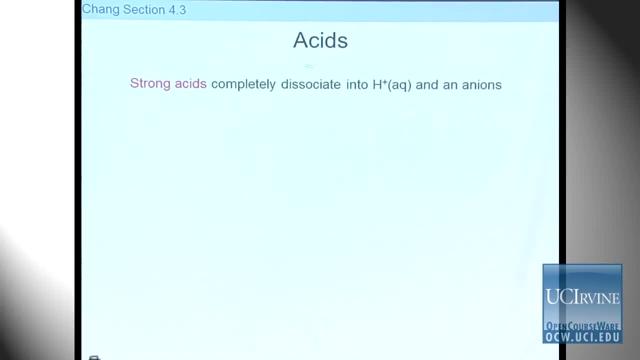 So strong acids are those acids that completely dissociate into H pluses and the correspondentào examples here: hydrog Iholderulan acid and sugar. hydrochloric acid is fully dissociated into H plus and the corresponding anion is Br minus. 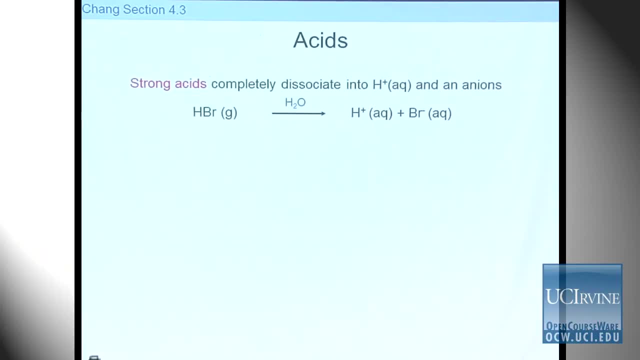 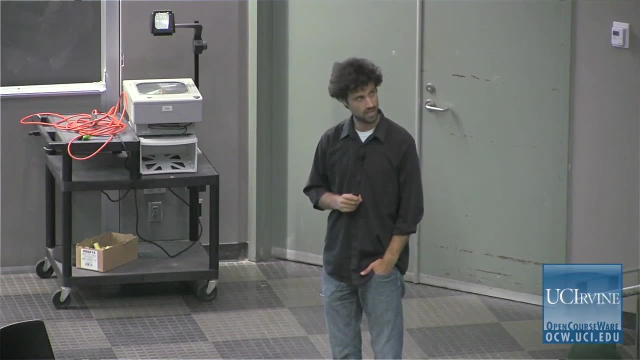 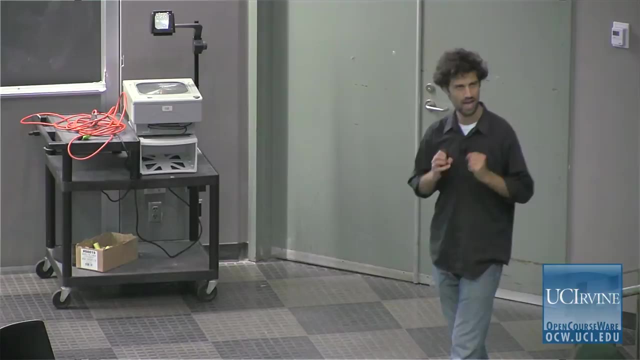 There's no HBr left. Everything is split. Well, the worst reaction in this direction is highly unlikely. The backward direction is highly unlikely. and we have already seen that there are six main strong acids. Okay, And here they are: hydrochloric acid, hyaluronic acid. 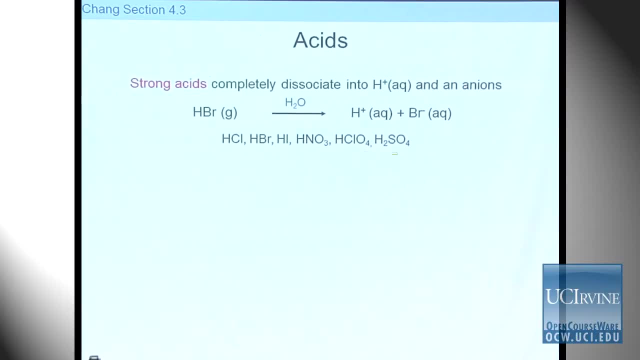 hydroiodic acid, nitric acid, chloric acid and sulfuric acid. Those are the acids that are classified as strong, So it also implies that if you see an acid that is not part of this list, try to Pickle it. 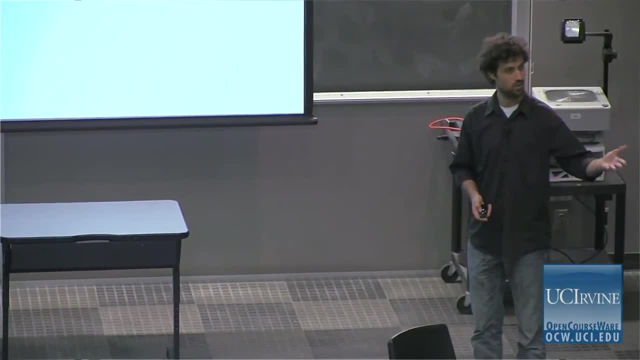 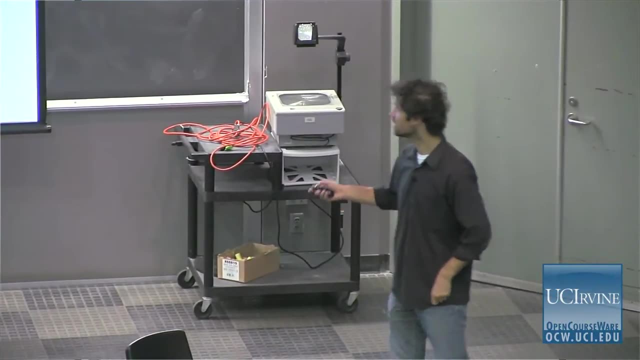 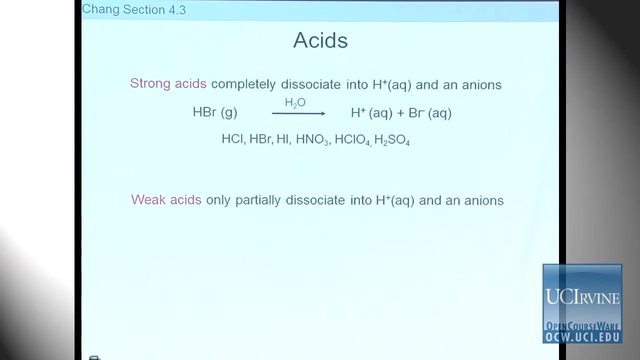 It is not media right. If it's still part of the list, you can actually impression it as a weak acid. So the weak acids are those acids that do not fully dissociate into H plus and the corresponding anions, meaning that there is a likelihood that H plus will go back to the anion and make use of the compound again, or the original compound again. Okay, Let's give an example. 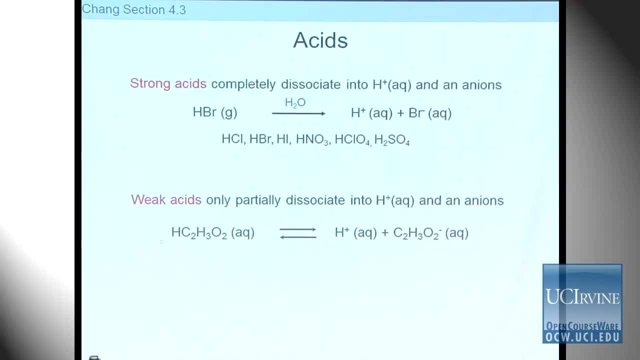 this is an acetic acid. this H can split off. We have seen this example already. This H can split off, Produce a H plus is in solution and it is an acid. This is the acetate anion, But the acetate anion can accept the H plus. 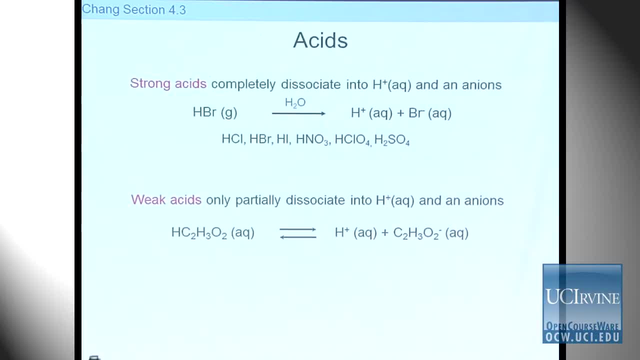 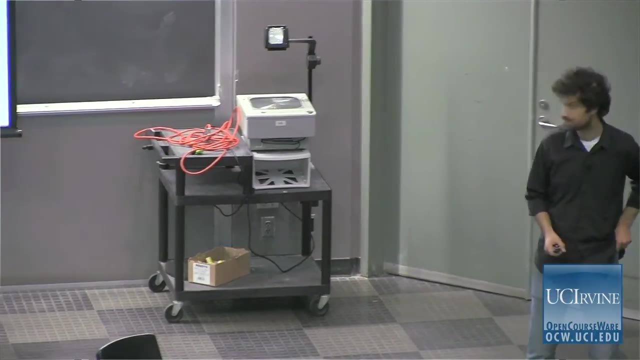 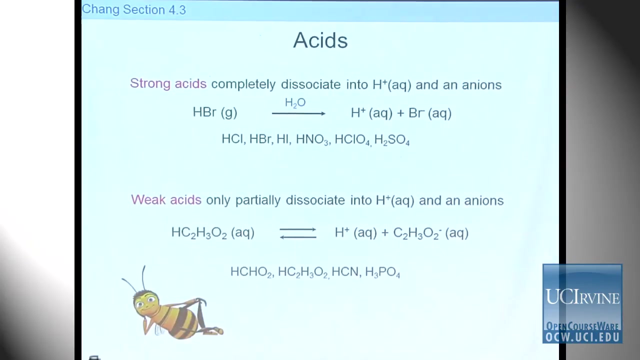 once again and go back into this species, the original compound. So at all times there's a portion that is always in this neutral form and then a portion that is split. Not everything is associated. We'll be part of that. So basically, every other acid that's not part of this list can be classified as a weak acid. Just let me give you some examples. 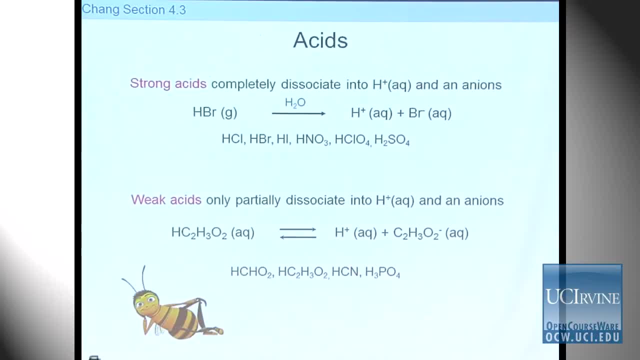 The simplest acid that contains that is basically a carbon-silic acid, is formic acid. Formic acid is the acidic compound in bee sting or, you know, in the antifungal. So that's simple silicon acid. Acetic acid- this is a hyperstenic acid. This is also a weak acid, And phosphoric acid, also a weak acid, is not part of this list. So anything else is basically a weak acid. 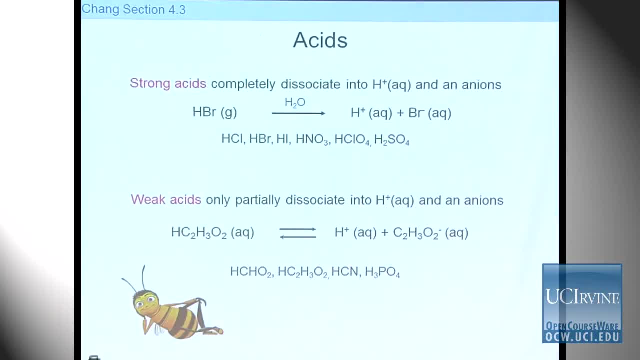 there are actually very, very strong acids beyond this, but we will not discuss those in other cases. okay, so we have strong acids and weak acids. we also have strong bases and weak bases, And so let's have a look at a couple of examples. 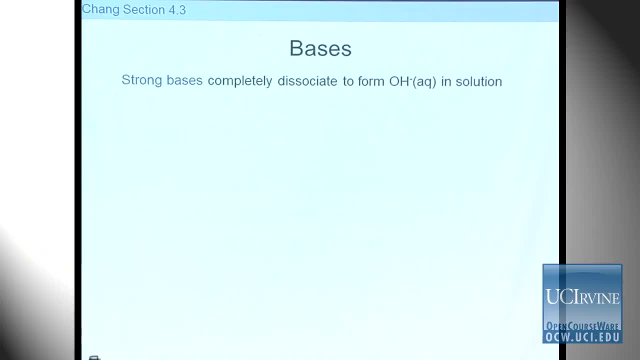 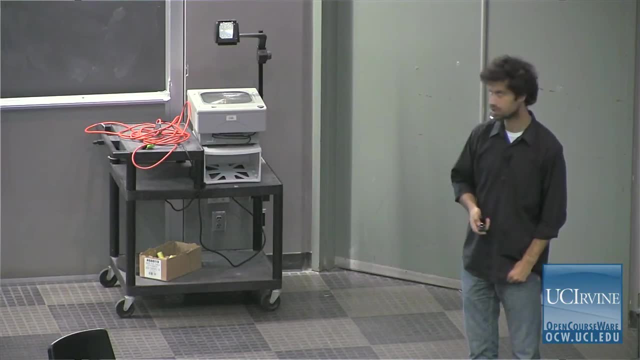 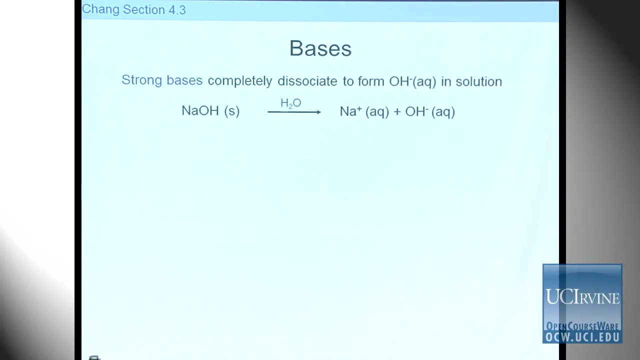 Strong bases, of course, are those that fully dissolve, fully dissociate in solution to form OH- in the aqueous solution. So the compound is fully dissociating such that it generates OH-. Here's an example. This is sodium hydroxide in water. 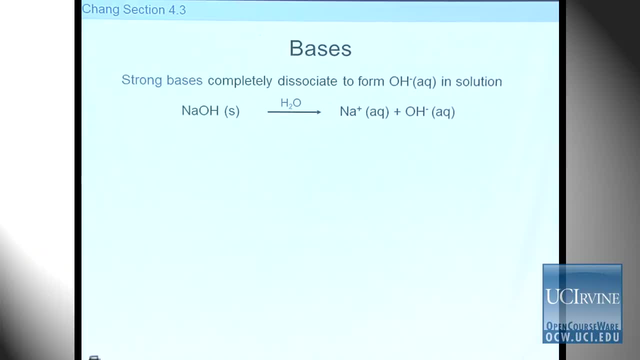 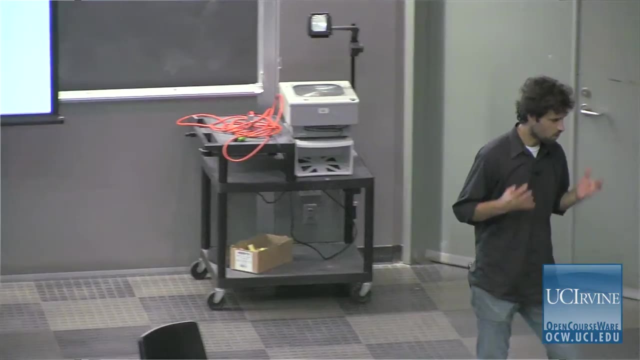 and it fully dissociates into sodium ions and hydroxide anions and this reagition is highly unlikely to happen under this set ratio. So this is a very strong base and basically most salts that contain the OH- the hydroxide anion- are strong bases. 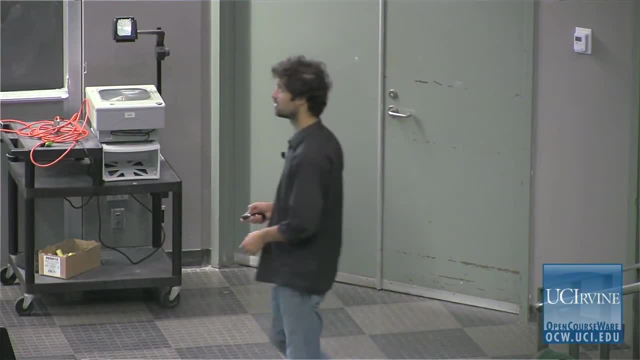 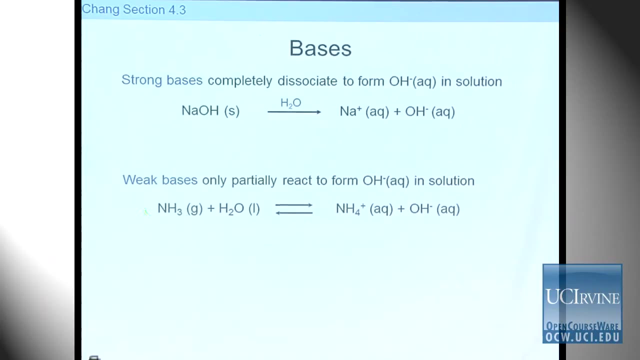 because it generates directly OH-. But there's more species that generate OH- under this ratio, and we've seen the example, of course, of ammonia Ammonia- sorry, This is the ammonia molecule. when it interacts with water, what it does? it can accept an H-crop for water. 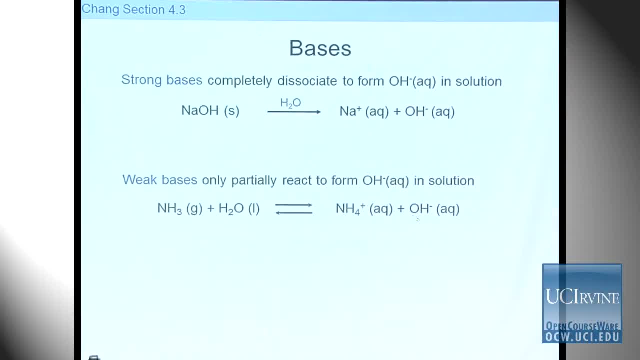 so it becomes NH4+ and the remnant, the water molecule that was missing in H+, becomes OH- and so effectively, it generated an OH- solution And hence ammonia is a base. It is not a base that contains OH- already Okay, But it does generate OH- if you put it in solution. 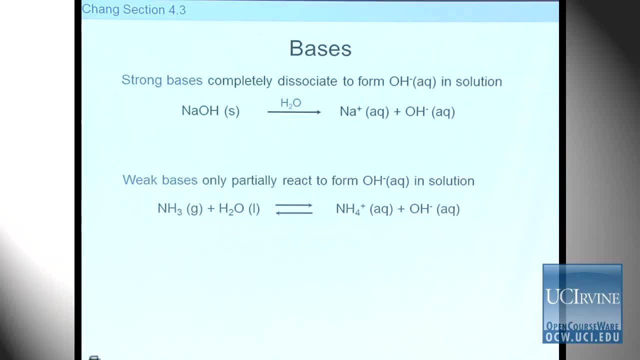 But of course it's a weak base. that means that the backup reaction is taking place and not all ammonia molecules are protonated into NH4+. Some of them will go back this way. Okay, so that's you know. we should be able to distinguish those four cases. 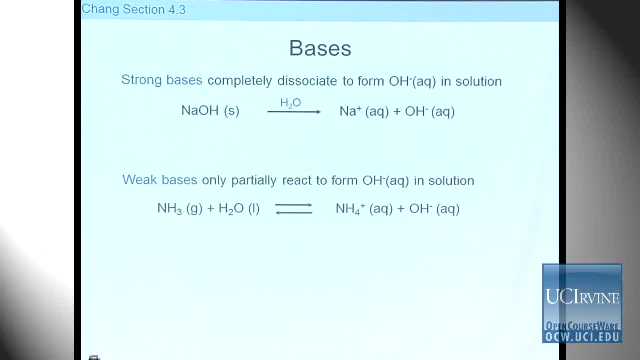 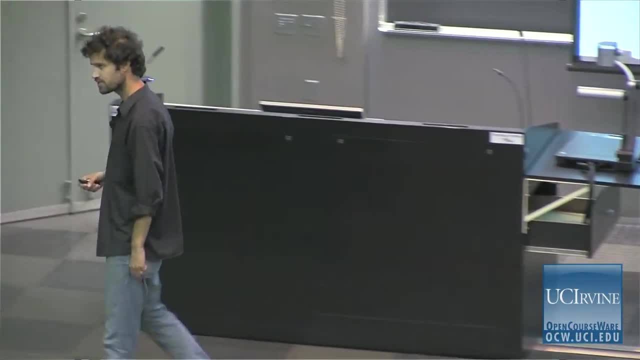 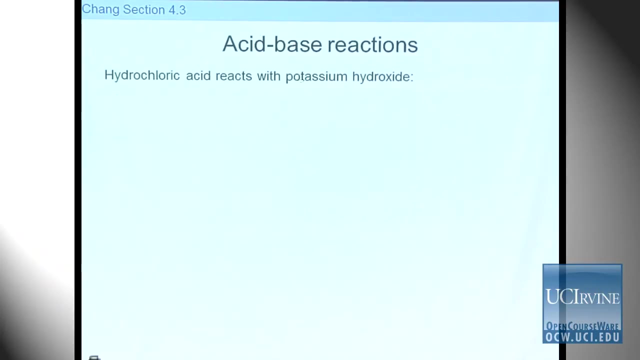 strong acid, weak acid, strong base and weak base. okay, so now we have these acids and bases. how do they react? Well, let's have a look at the section the reaction. isatti teen positions, which a win einsel on my mind. 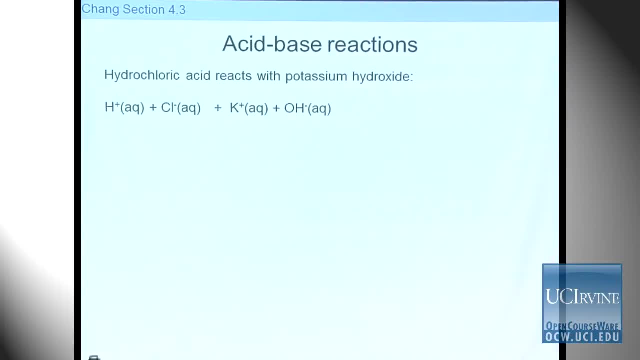 that's fine. So this is. I'm writing this out in terms of the complete ionic equation. So this is the acid, because this is the H+ and the base in the solution is the OH-, And so what will happen is: what do you think will happen? 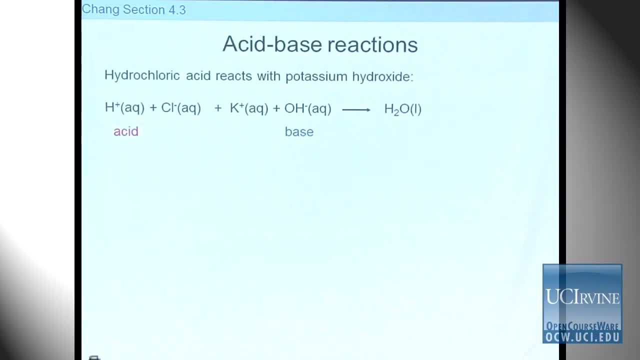 This H+ will go there right, So they interact, form water. so the H+ will go to the OH- to form water, and then these two guys are left. Nothing happens to them, they just stay in solution K+ and CO-. 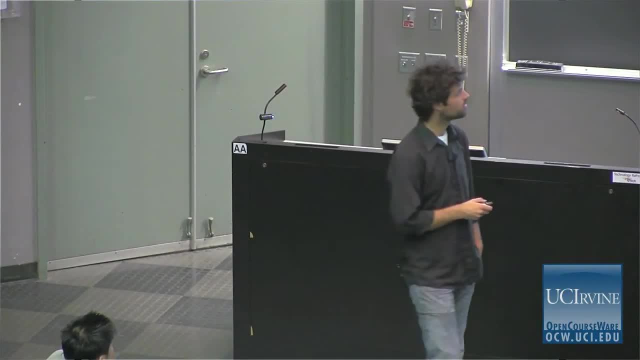 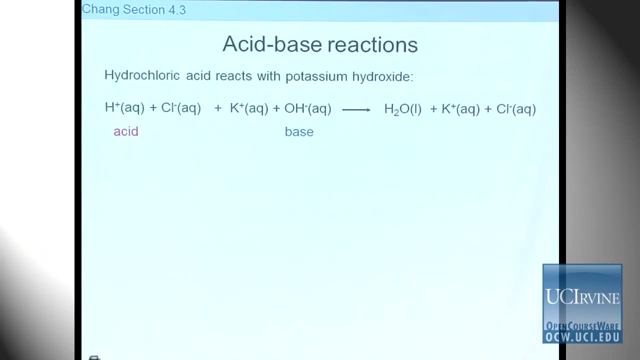 they will stay in solution, will not form a new compound and therefore these guys are called the spectator ions. So I can again use the same trick that we learned about last time: cross out those spectator ions and I'm left with a net ionic equation, which is: 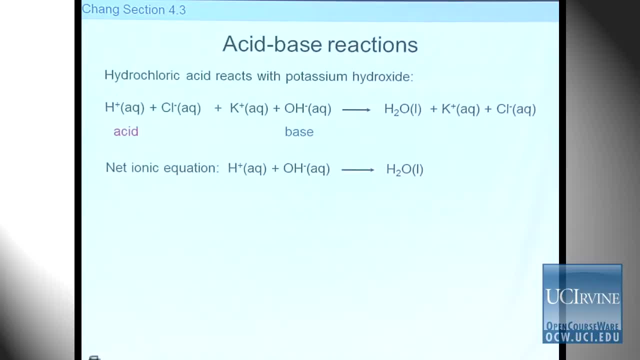 H+ interact with OH- to form H2O. This is the basic, the most fundamental acid-base reaction. H+ is in solution, interact with OH- is in solution and they form a water molecule. This is the most fundamental acid-base reaction. There's more time. 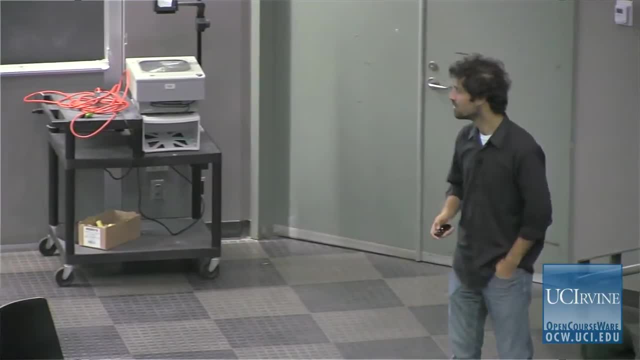 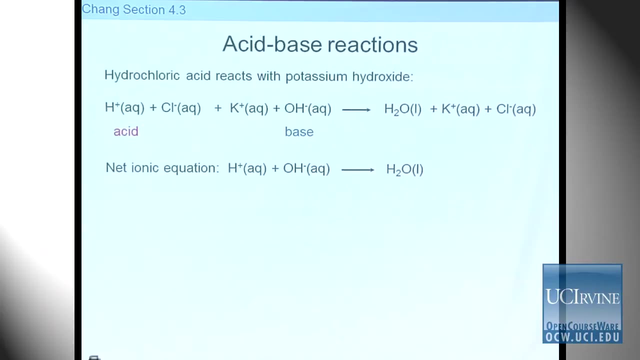 This is the most fundamental. Okay Now, if you have the very special situation, you have exactly the same amount of H+ as OH- is in solution. So the same amount of moles of H+ and the same amount of OH-. they will combine to form a water molecule. 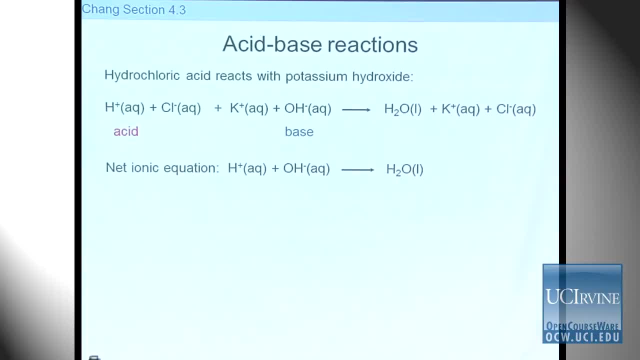 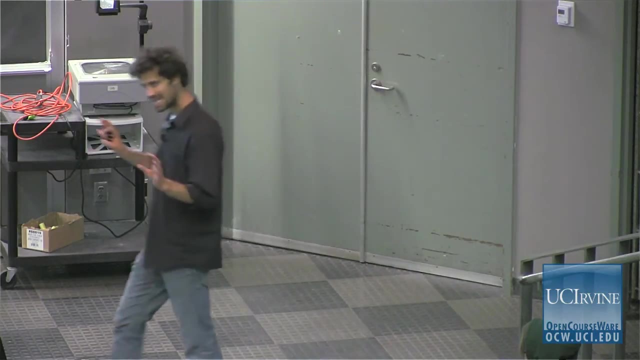 And if you do that, you have no H+, no OH- left. so you have neutralized my solution. Ok, So neutralization reaction is when the amount of base reacts exactly with the amount of acid in solution neutralized, exactly the amount of acid in the solution neutralizing the acidity. There are technically no H pluses floating around in the solution, All taken care of And the solution is called neutral. You'll learn in the camera to see what neutral really means. okay, Neutral means there's no- all the H pluses are gone because you have to sell deprotonation of water, but beyond that, all the H pluses are gone. So the solution is called neutral. 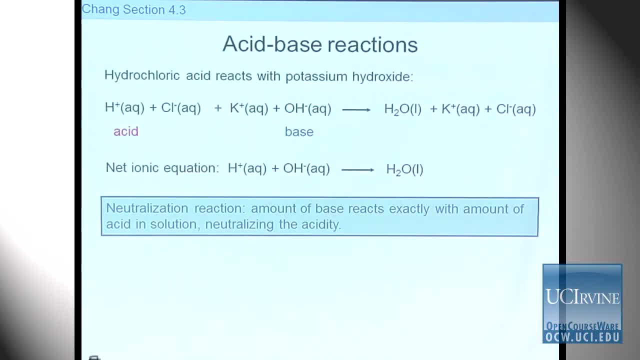 So, for all intents and purposes, you consider the solution to be fully neutral. Let's look at another example. Here's one: Aqueous sodium hydroxide is reacting with acetic acid. Now, acetic acid is not a strong acid. 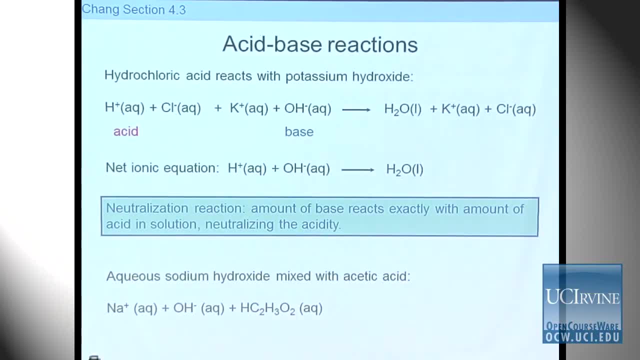 This one is right, This one is not. So here it is. This is a complete ionic equation. again, Sodium ions, hydroxide ions, that is, sodium hydroxide. This is acetic acid. Acetic acid is actually a compound. 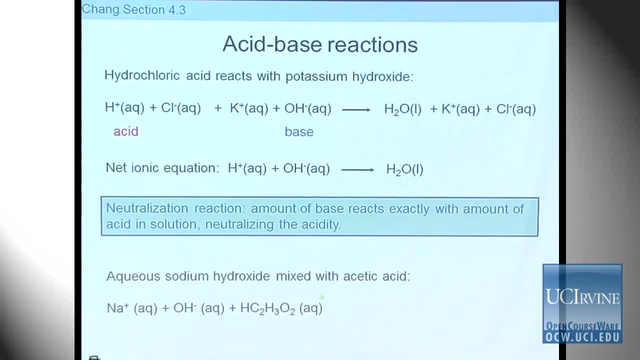 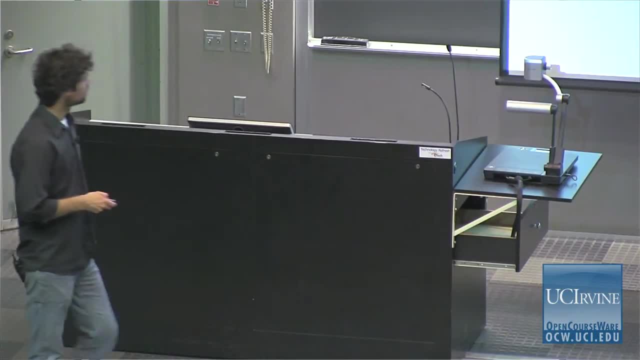 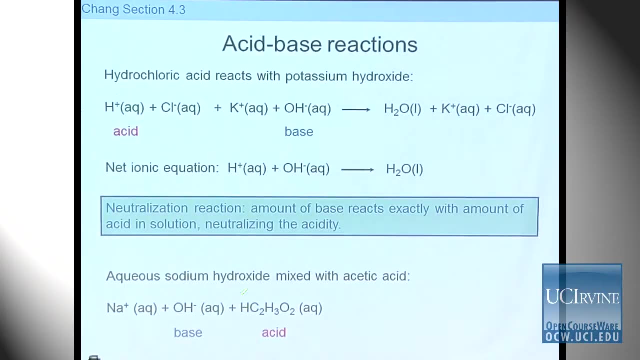 where H is attached- this is a molecule that's dissolved in the solution. So this aqueous means that the solution doesn't necessarily mean that it's split already. This OH likes to pluck out this H from acetic acid. So this is the base and that is the acid. 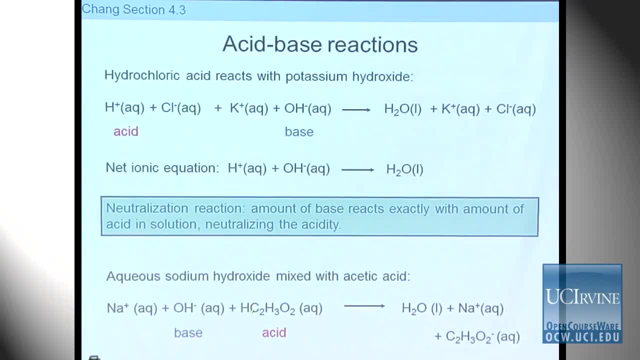 and they interact very strongly. In other words, all the H's will be plucked away from this weak acid to form H2O. Sodium is the spectator and the rest ion is the acetic ion. Now, interesting situation here. This was a strong acid and a strong base. 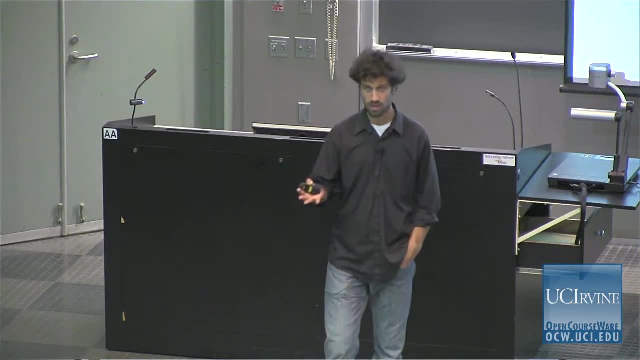 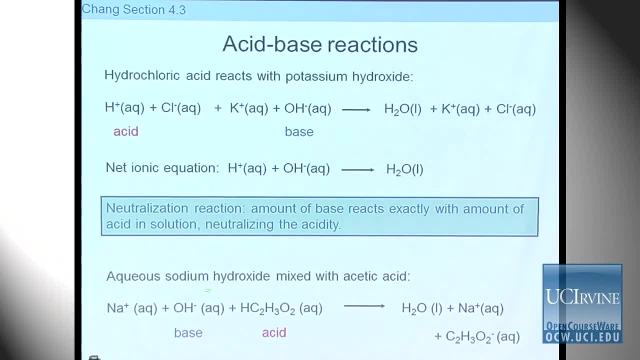 Zero, Zero, Zero, Zero, One from each One more equal. that One is in it. No, No, No, No One is in it. No One is in it. No, No, No, No, Nooo. 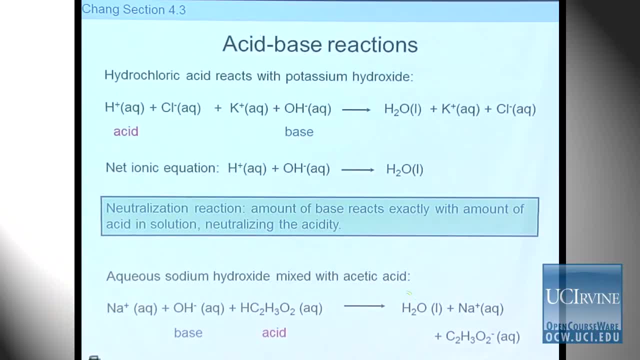 because it is much less favorable to give up the H from the H to rho, sticking again to the acetate to form OH- OH- will immediately go back this way. So as soon as you have a strong acid or a strong base in solution, the corresponding reaction will most likely be not reversible. Only if you have weak acid and weak bases. both then you have a reversible reaction. 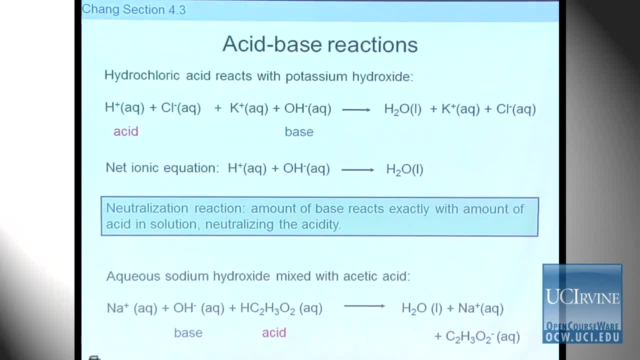 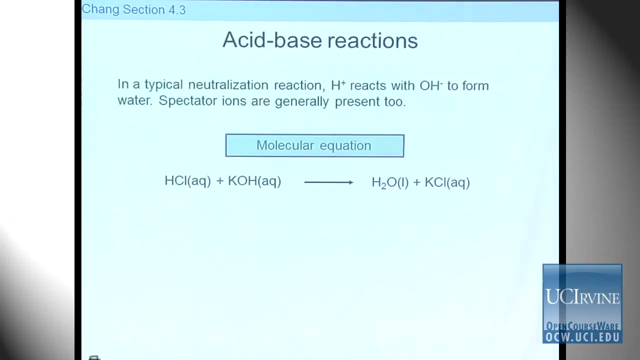 but as soon as you have a strong acid in there or a strong base, you can consider this reaction to be unidirectional: All the H pluses and all the H minuses will be consumed. Okay, Let's say it one more time, in a different way. We saw this reaction on the previous slide. 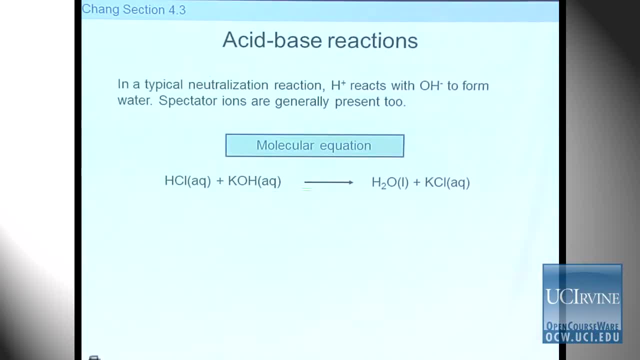 We saw HCl and potassium hydroxide. Now I'm writing it in terms of the molecular equation. This is just another way of writing the same equation. HCl is now written as a molecular compound. aqueous means it's fully dissolved, right? 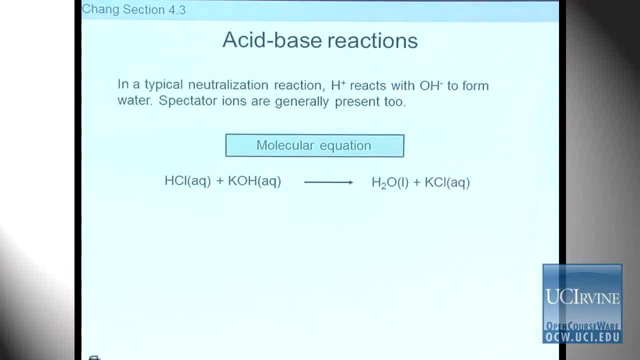 KOH, aqueous is also fully dissolved. If you write it like this- and I've seen several people do this- okay, Don't write a plus here and a minus there, Because this compound aqueous means it is already dissolved and it is understood that this is split. 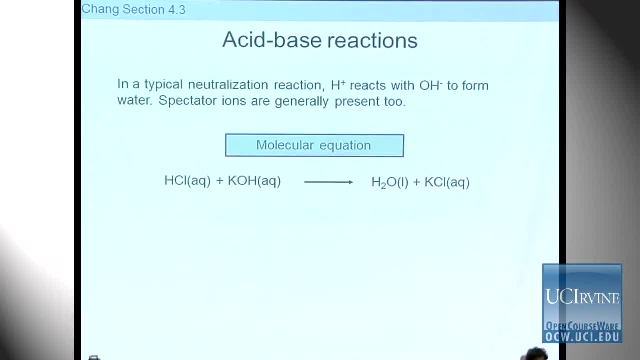 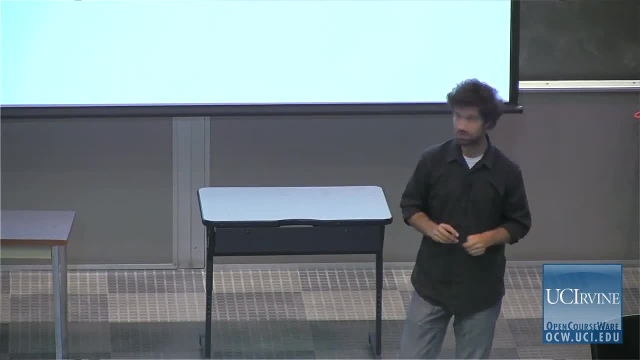 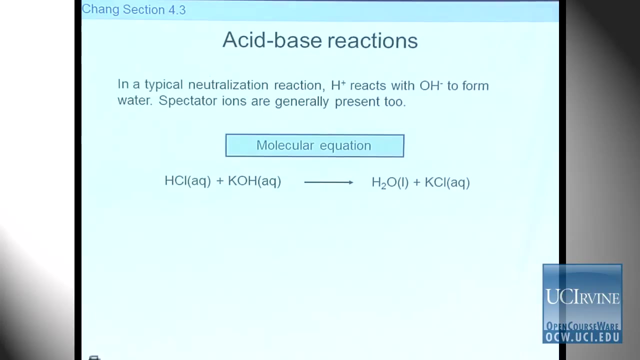 If you split it, you have to split both and put the aqueous sign in both. Don't smoosh it together and then squeeze a plus and a minus in there. This is not a proper way of writing this compound. You either split it fully or you leave them together without showing the charges. 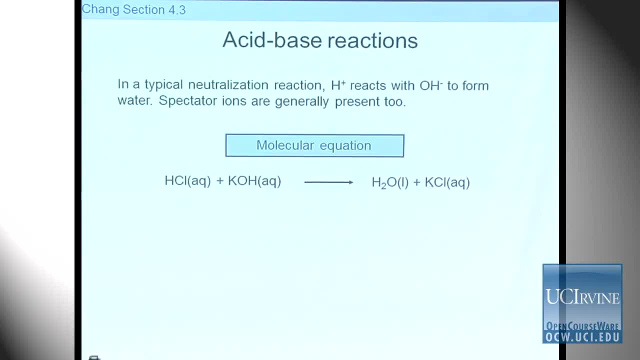 So we saw what happens. The H plus interacts with the OH forming H2O, and KCl is the other compound that is still in solution, fully split. but in the molecular equation they don't show that they're separate. They don't come together without showing the charges or the ions. 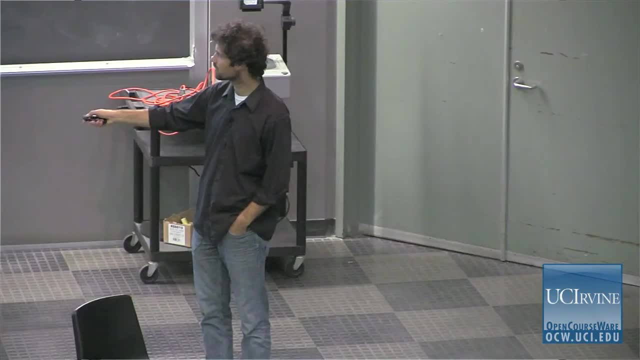 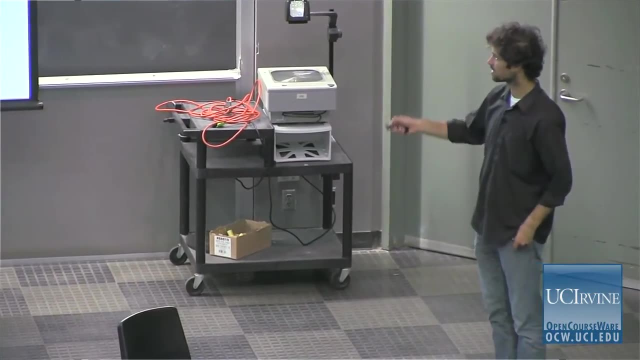 This was the net unit equation. We concluded: H plus OH minus H2O. all the rest ions are conflicted ions that are taken care of. In a nutshell. Again, this is an example of a fundamental acid-base reaction between H plus and OH minus. 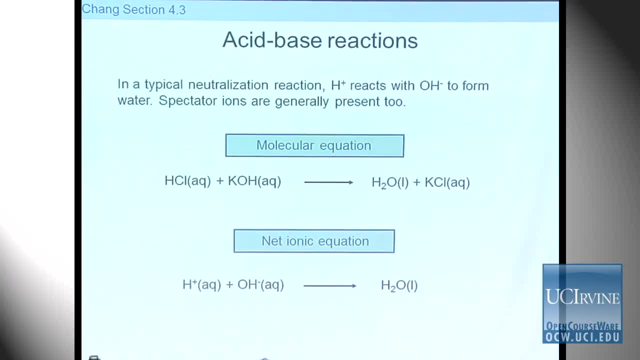 Okay. Well, we're done with that. Thank you for your attention. See you next time. Let's look at one more example and try to write these equations correctly, and then we'll jump into the calculations. Okay, So I have here a reaction. 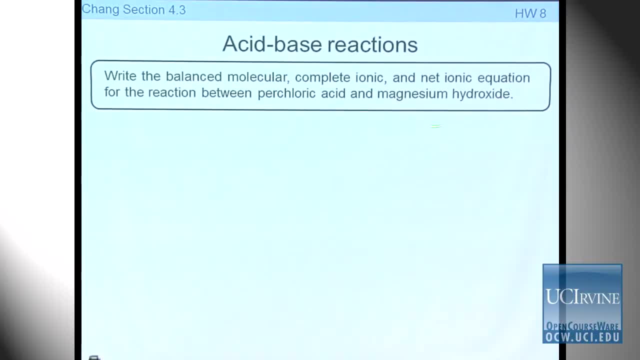 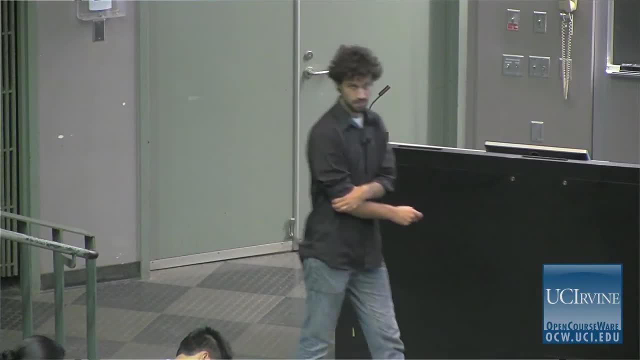 it is perchloric acid and it's interacting with magnesium hydroxide. Perchloric acid is a strong acid, but magnesium hydroxide has a very strong base, so this will definitely be a unidirectional reaction In the molecular equation. 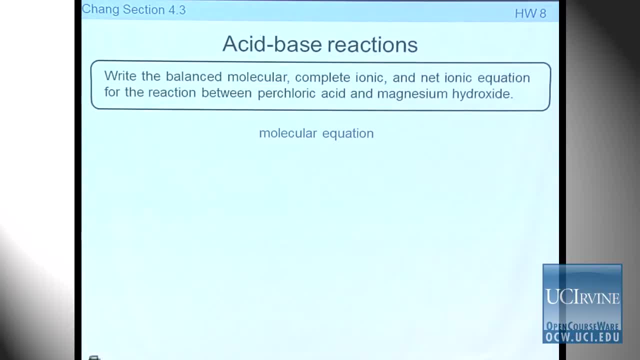 what I do is I'm going to write down 10-12,, 40-50-40-45-50.. full compound: Chloric acid is here, HClO4 aqueous. that is the molecular compound. don't show the charges here. 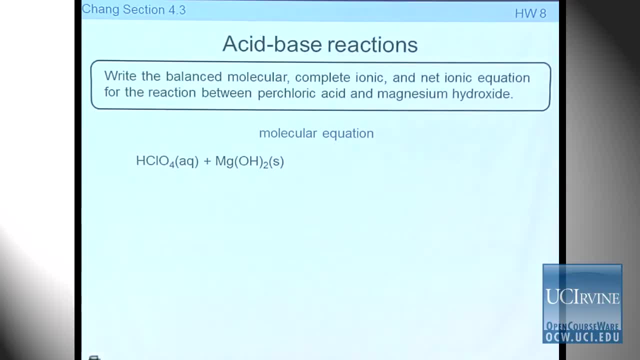 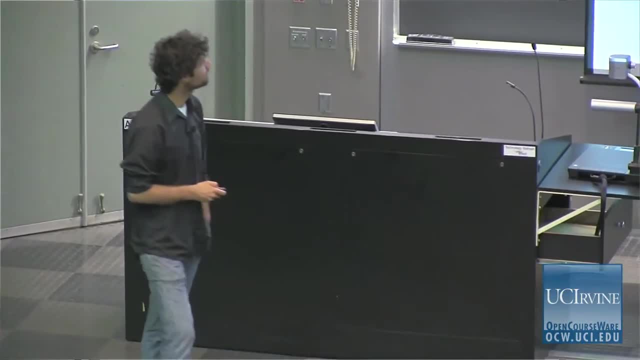 Okay, Once again, And this is magnesium hydroxide: Magnesium with two hydroxides attached, because magnesium is 2+, So you need two hydroxides to make it neutral. Magnesium hydroxide happens to be a solid That's not given here in the question. 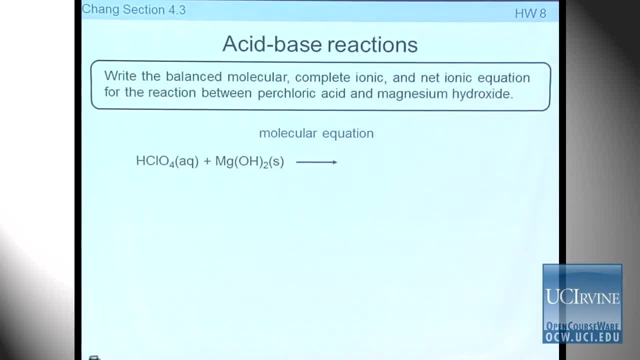 So I put it here anyway. All right, What's happening? Well, this is OH-, That's a strong base. H+, of course, is interacting with it to form water, and the other two that are still in solution are the magnesium ions. 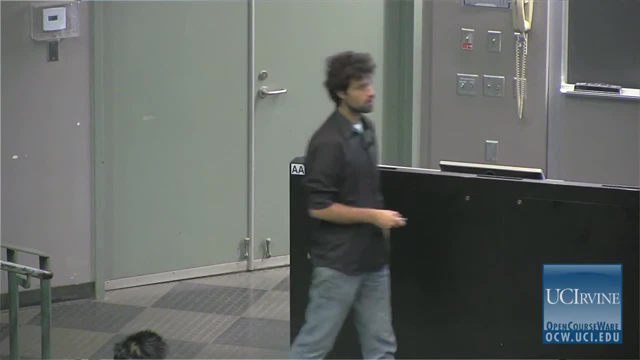 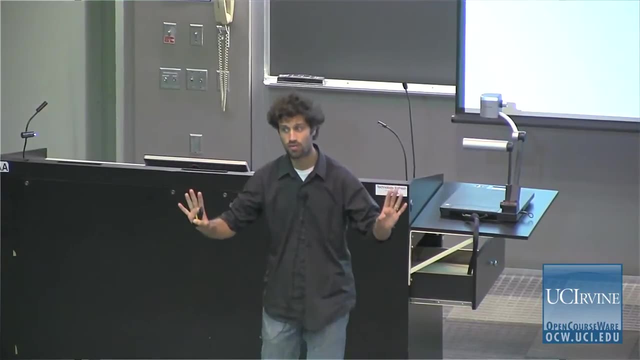 and the perchlorate anions, And the way to write that in the molecular equation is to put them together as a compound, But it's understood that they are fully dissolved into ions. There's one problem with this, and that is it's not balanced. 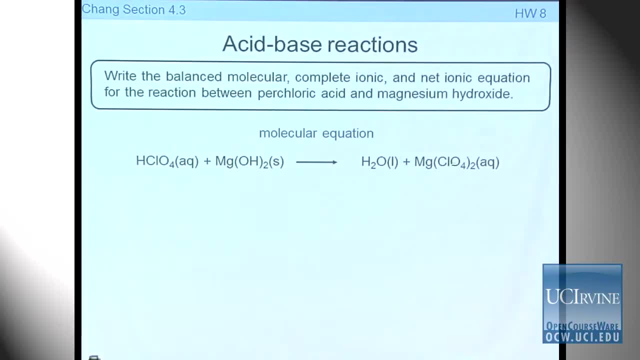 Okay, You can see that immediately, because I have two. I need two of these perchlorates for magnesium to make it neutral. I only have one here, So I need definitely a 2 there. I put a 2 there, and if I do that, I have an issue with the number of H's that I use. 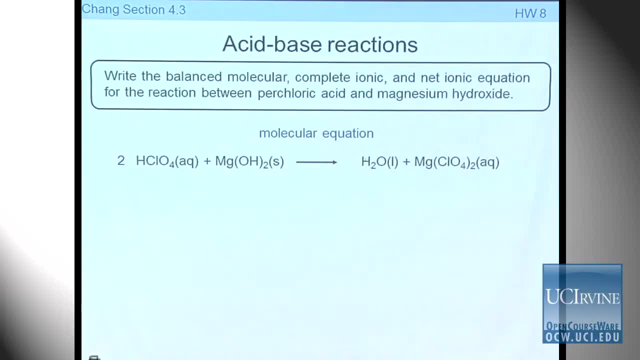 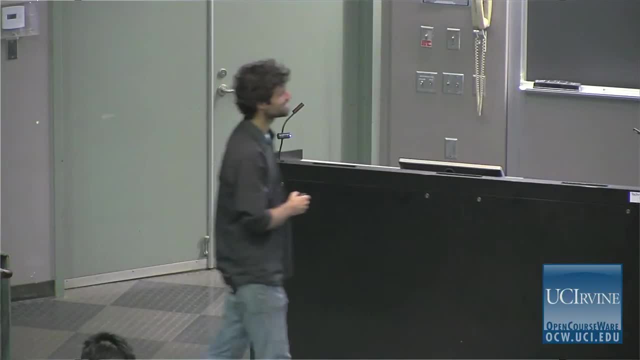 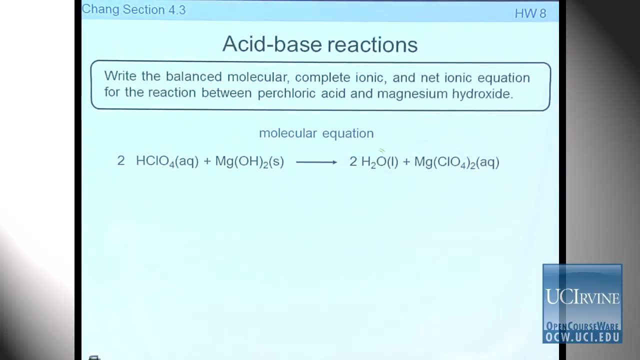 there's two here and there's two there, but there's also another 2 there, So I need a 2 in front of the water and let's check if I do everything right now. two oxygens, two oxygens, four H's, four H's and two perchlorates. two perchlorates. This is right, This is balanced. 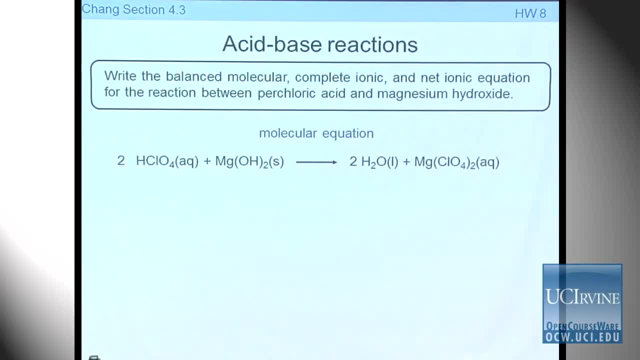 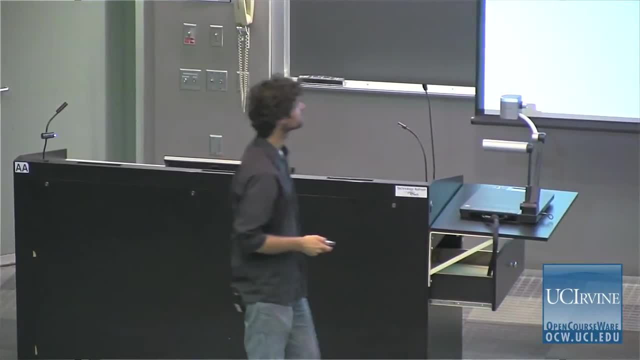 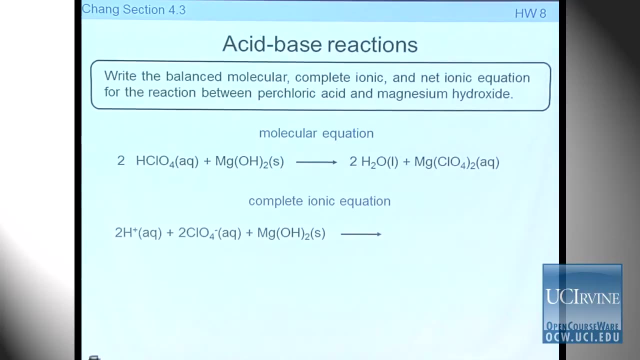 Make sure you balance the equations right, because if you do calculations with the equation that is not balanced correctly, you get very wrong numbers because you finished with a more or less Okay. The other part of the question was to write the same equation in terms of the complete ionic. There we go. 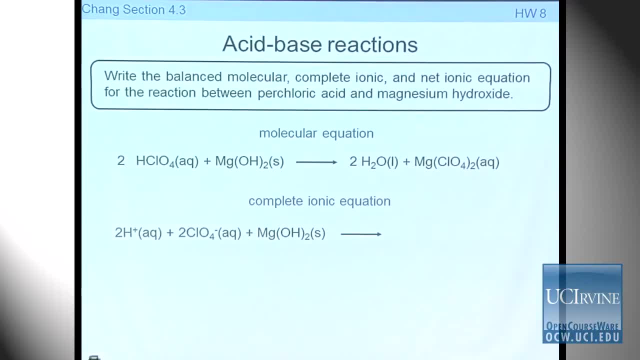 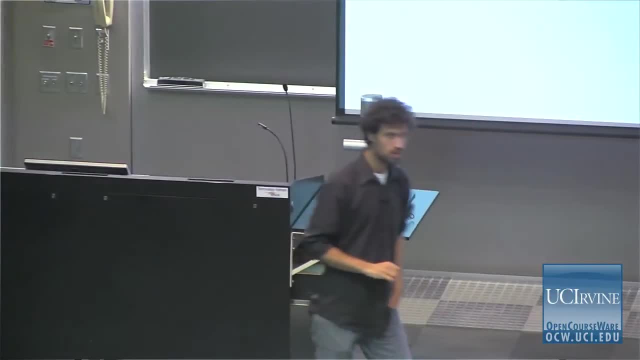 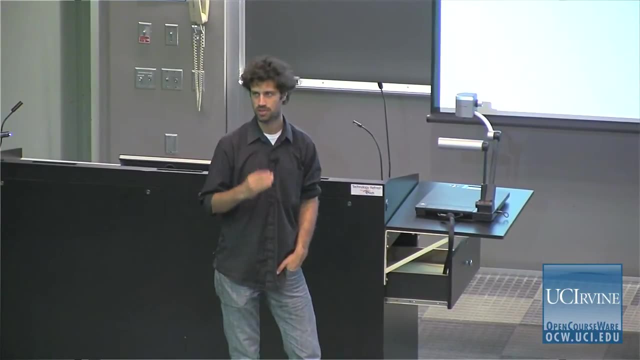 What I do is I just split this compound into ions. I will show you an example- I think on the next one there. so from previous exams where people are trying to do this and a common mistake. I'm not sure exactly where the mistake comes from, but 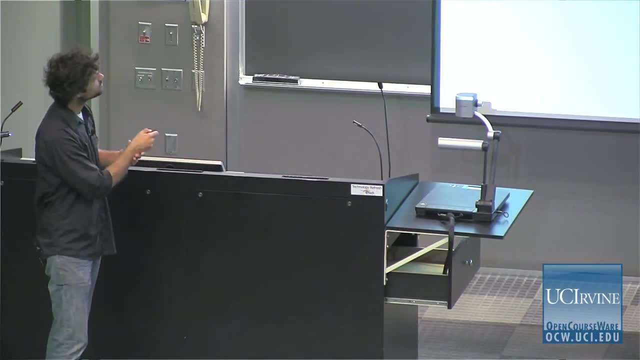 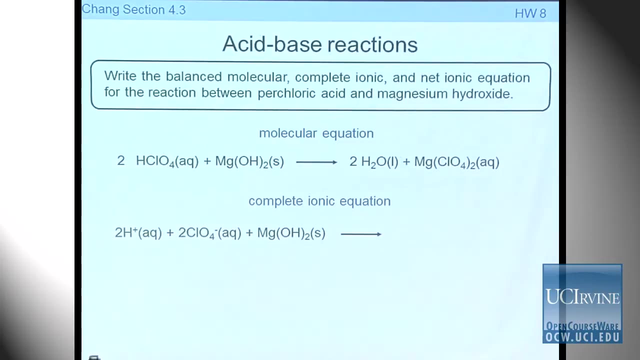 about 10% of people do. this is when I ask you to split this molecular equation into a complete ionic equation. they take each element- H, Cl and O- and split them all up into aps, dissolved elements. I've never seen this anywhere in the lecture in the program, but some people do that. 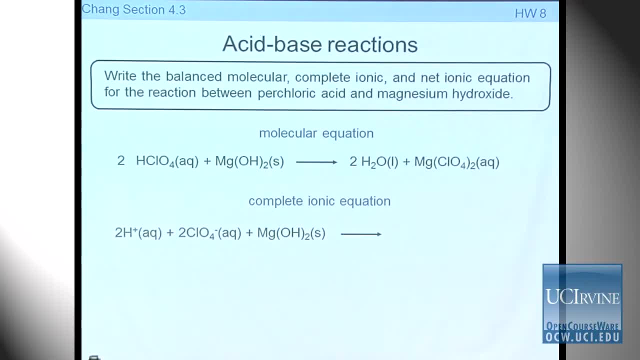 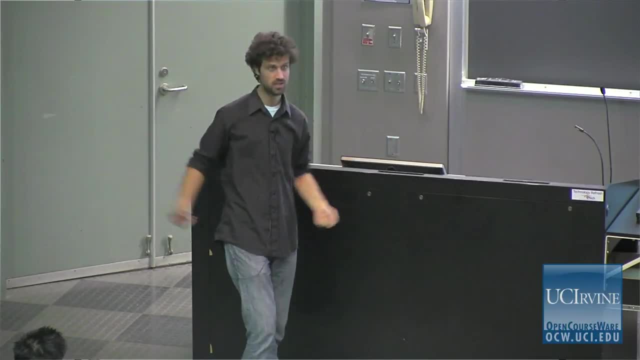 I would like to make sure that you are not one of those folks. If you split something into ions, you can split it into ions. you don't split it into all kinds of elements, right? That's not the idea of a complete ionic equation. 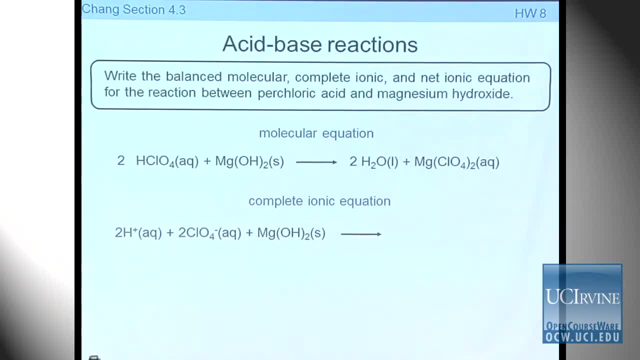 so the ions in perchloric acid are H+ and perchlorate. Perchlorate is an anion. This is the anion. You don't split the anion again into elements: two H pluses two perchlorates. 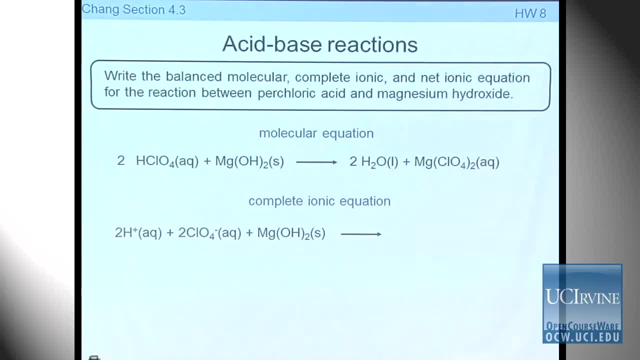 magnesium hydroxide is a solid, so I don't split that in the complete ionic equation because these are bonded But they're not fully dissolved in solution at this point. However, when this H plus is attacking the OH minuses, it will fall apart. 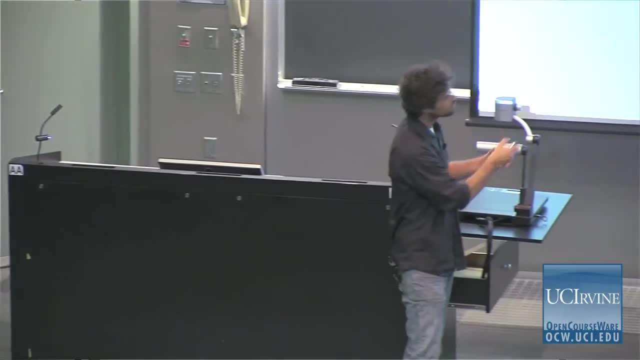 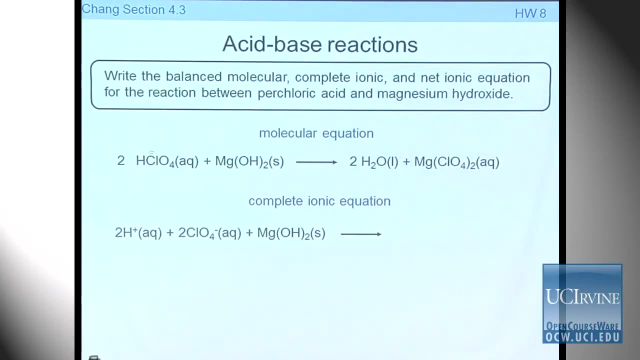 this is kind of like all of you understand. the fact that this is an S doesn't mean that it doesn't react. it does. It's like you throw some solventeure up in a solution. the H pluses will directly attack the OH minuses in the lattice, In the solventeure lattice. 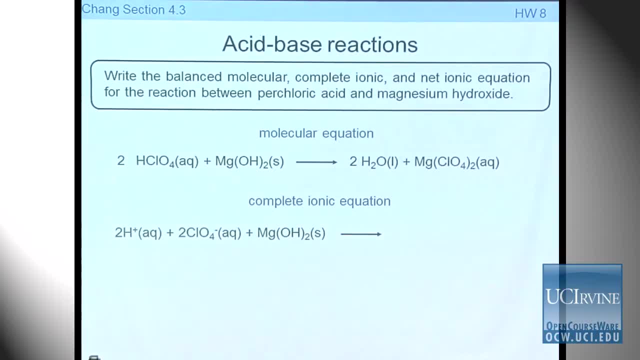 and pluck away these OH minuses, bring them into solution, and then it will fall apart, Which is pretty easy, doesn't it? It's pretty easy, isn't it? We will see how that works in the future. the rest, ions magnesium, are floating around here, So what we have? 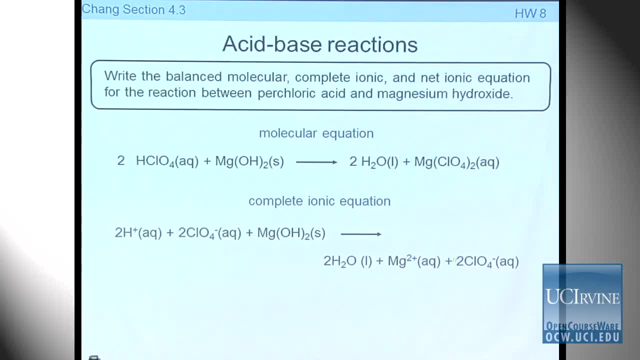 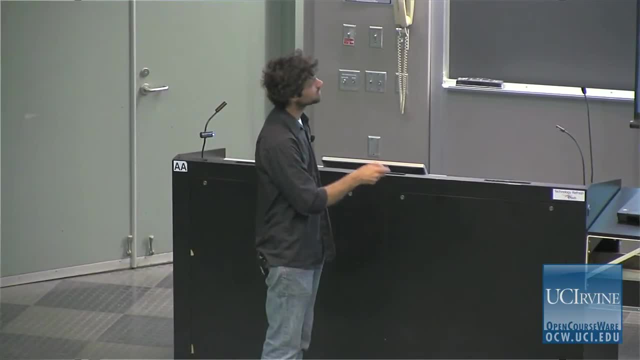 we generate two waters. we know that from here. magnesium ions and the rest ions- the spectator ions- are perchlorate. The last one is a net ion equation. the only thing you have to do is strike out all the spectator ions. This is a relevant example, okay. 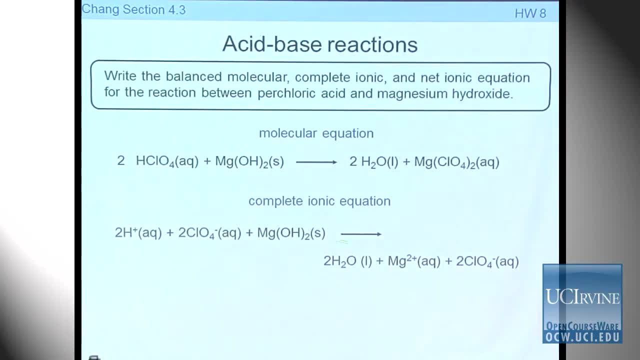 because you are not striking out magnesium. magnesium appears here, but the ionic form of magnesium is not on this side, so you can't strike out magnesium here and take it out here and- no, it doesn't work. if you cross out spectator ions, they really have to be ions that are fully dissolved and separate. Then you cross them out. 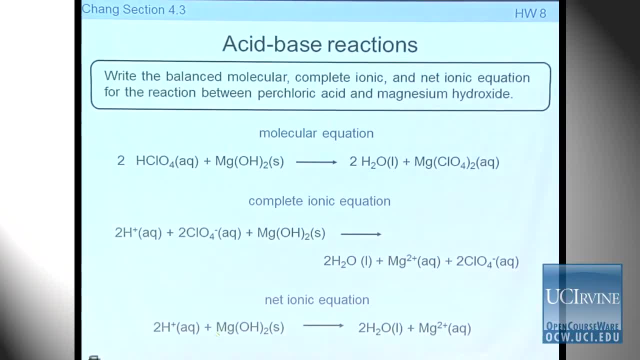 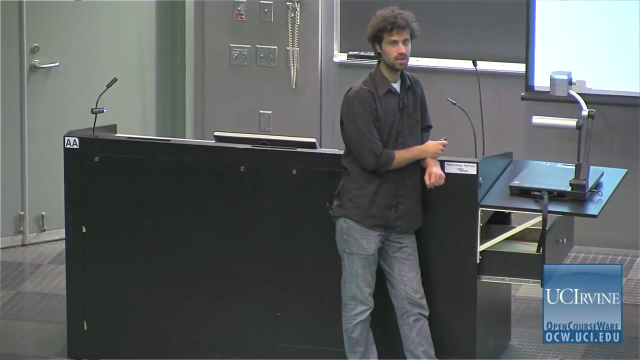 so the net ion equation is this: H+- magnesium hydroxide is fully here. H2O- magnesium 2+. it's there, not crossed out? the only thing that's crossed out is perchlorate preserves appearing here in the same form as it appears over there. Is that clear? Yes, 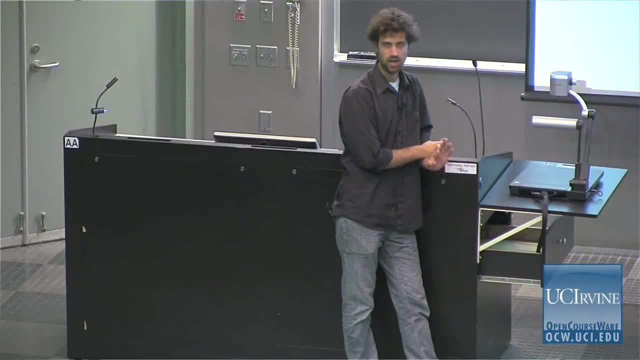 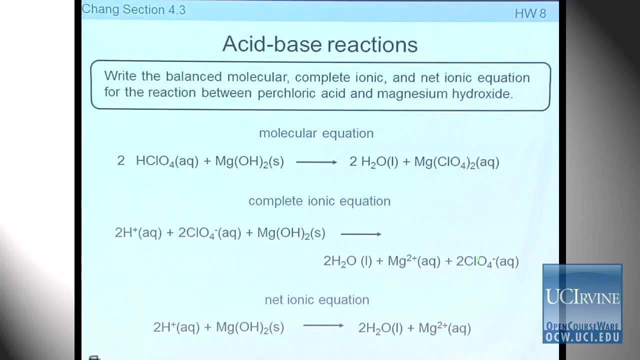 Magnesium hydroxide is a solid. The magnesium ions are not dissolved in solution on this side of the equation. Only after the H plus is reacting with it they become available as ions in solution. So you cannot cross out this ion on this side. 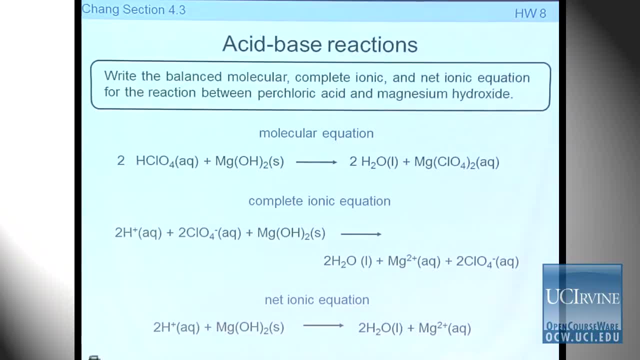 with this bonded ion in the lattice. Okay, You cannot do that. You can only do it if it's a real spectator ion. A real spectator ion is if it appears fully dissolved in solution on one side and on the other side. Now you see this equation here. even though there's a plus here, this is a little awkward. 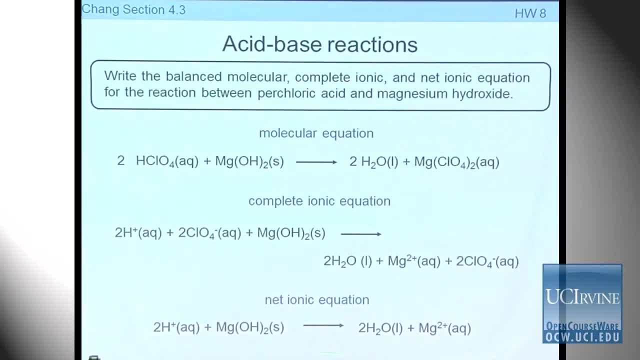 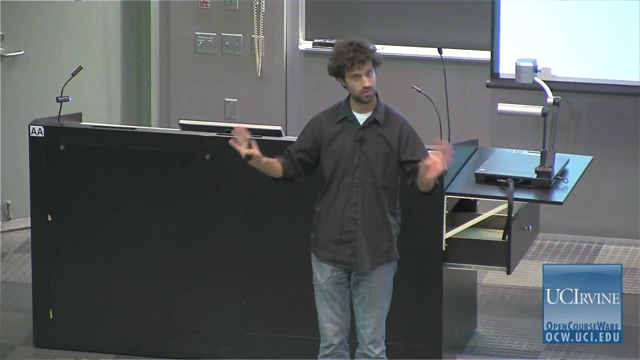 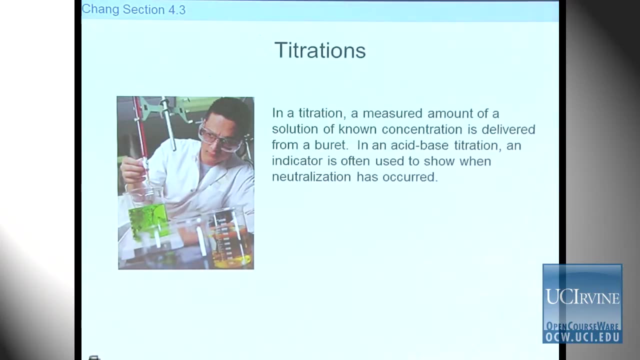 there's also a two plus here. Two times positive charge is two plus and then two plus. This equation is fully balanced in terms of elements and the charges. So this is a perfectly fine, balanced nebule equation. Okay, Let's move on to the following. 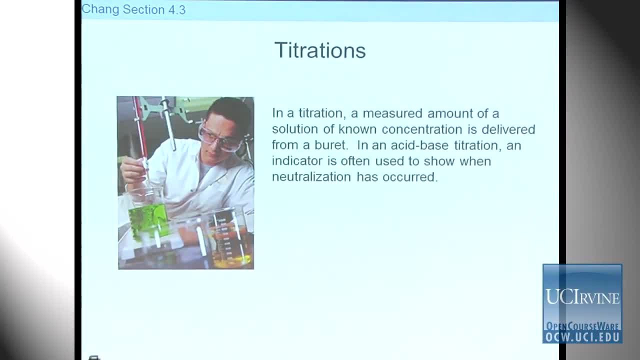 This person looks like a very capable chemist and he's doing something here. He has some red solution here, opens up a little valve, it drips into here and this is beautifully green. this is wonderfully yellow, Actually. I mean, you are in the lab. 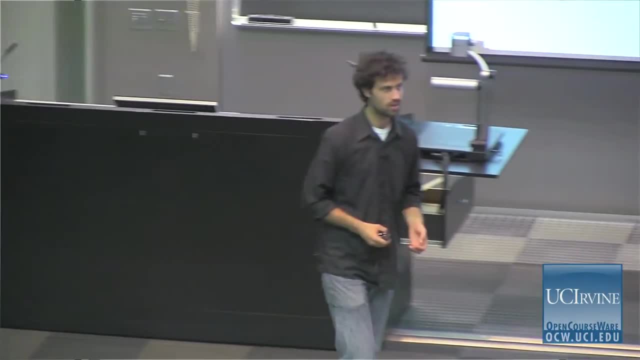 I mean, you've got somethingyes really eatable. You know that's life. No, frankly, that is, that's just easy. And for real, most solutions of this boring, you know, transparent, can never work all day long, But for photographic. 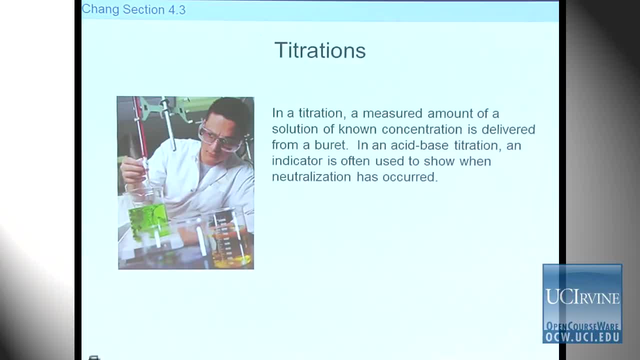 opportunities- they are beautiful- to Tim Alex, Just to get them excited about chemistry. So what is this person doing? He's doing a titration. What is that? Well, you have this thing here, a barrette, and he's dripping something of that stock from sitting in here. 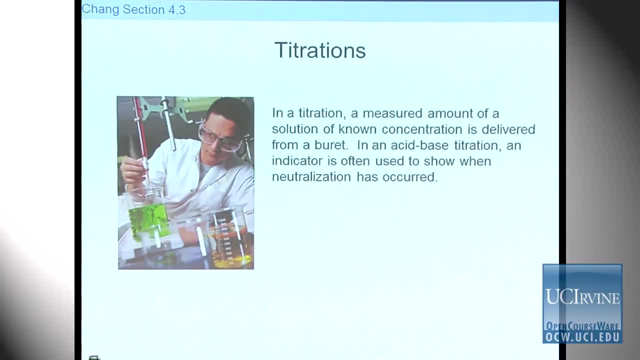 in this beaker till the moment when a certain reaction is taking place, until complete, And he can read out on this bread, which has an indicator on it, how much he used, and he can use that information to quantitatively determine how much of the other stuff is sitting in this beaker. So it's kind of a quantitative analysis method to find out how many ions of a certain kind are in here. 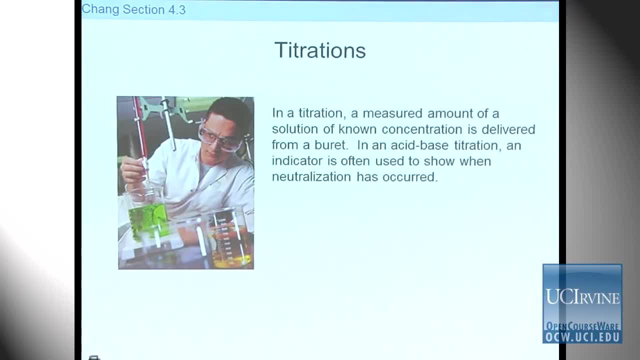 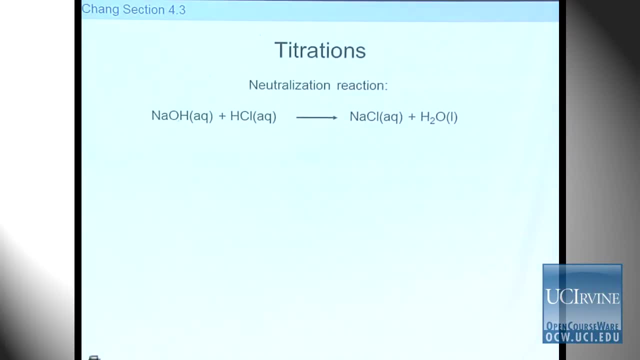 So, in terms of acids and bases, this is typically what you use for a neutralization reaction. Let's have a closer look. Here's one: NaOH sodium hydroxide- this is hydrochloric acid. this is the two products that form water and sodium chloride in solution. 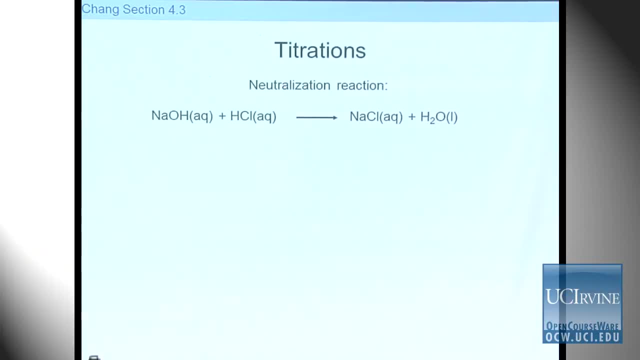 OH is interacting with the H from the HCl forming water. So you can do this reaction in the following way: I have, in this particular case, HCl, the acidic solution, in my beaker and I'm dripping with this barrette the NaOH. 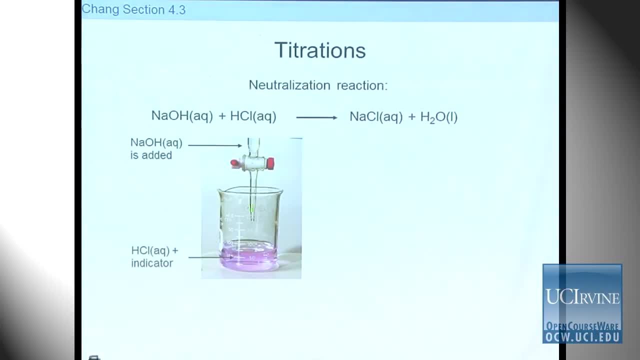 That's the basic solution And I can control how much I add. so I know exactly how much I add. I know the molarity of this. think about it. You know the molarity, you know how much volume you apply. the volume times molarity is exactly how many moles you added. 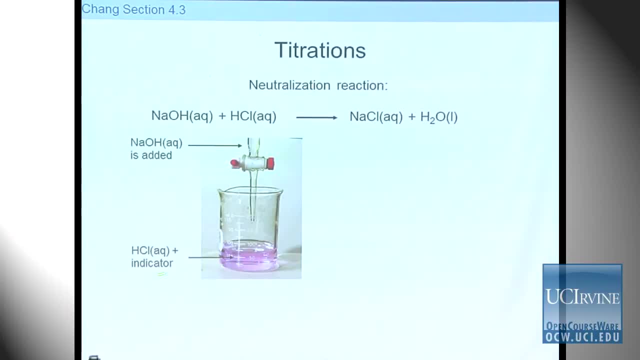 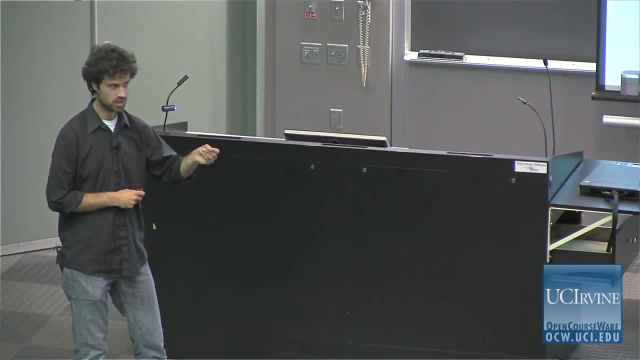 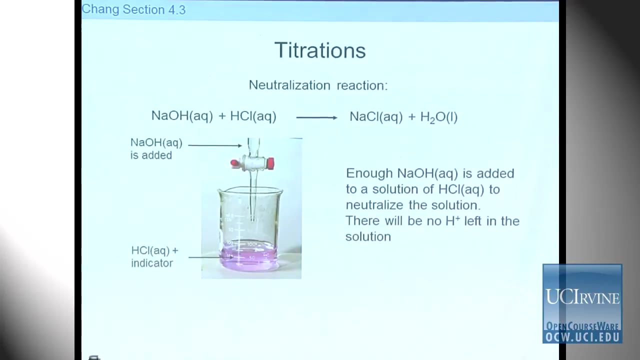 And you can see when something happens here. Now, importantly, there's also an indicator, and the indicator tells you exactly when the pH or the number of H pluses. So this will tell you something about whether the reaction is completed or not. There's actually a little movie here that I have. 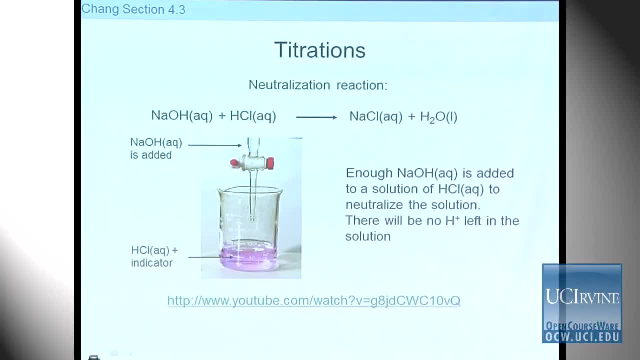 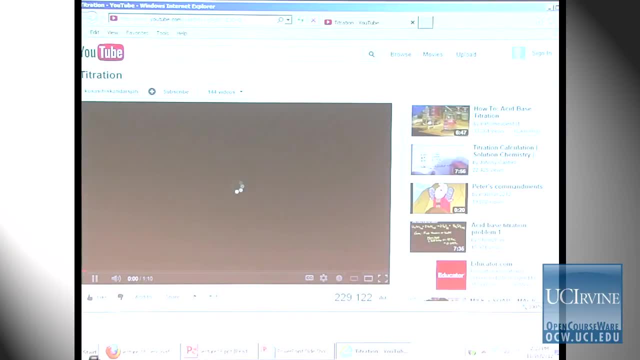 Let's play that, See if it works. All right, I don't know why it doesn't play. Oh, there it is. A titration is a controlled acid-base neutralization reaction. Twenty milliliters of hydrochloric acid of an unknown malaria. 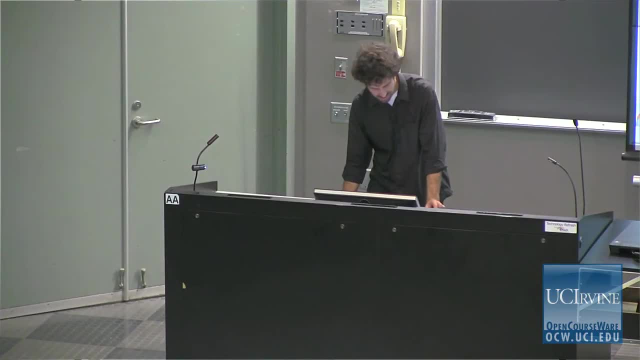 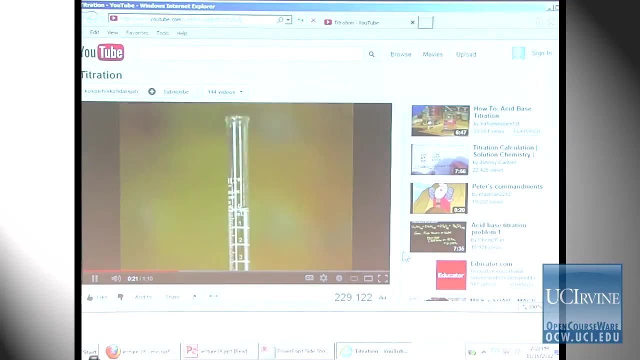 Oops, sorry. Two drops of indicator dye are added to the acidic solution. This indicator dye is clear in acidic solution and pink in basic solution. The burette is filled with a sodium hydroxide solution of known strength and an initial reading is taken. 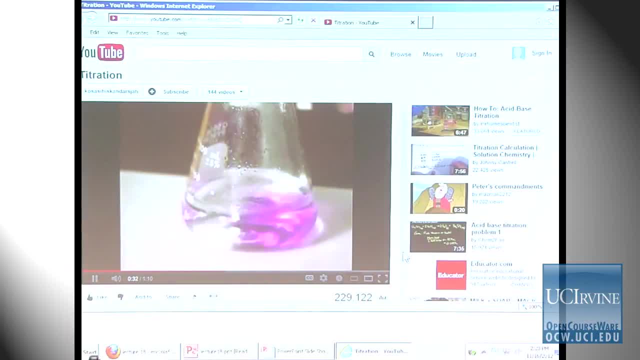 The base is added to the acidic solution until the solution stays a slightly pink color. At this end point a final reading is taken. The moles of base added equal the moles of acid present. This same reaction can be followed using a pH meter instead of an indicator dye. 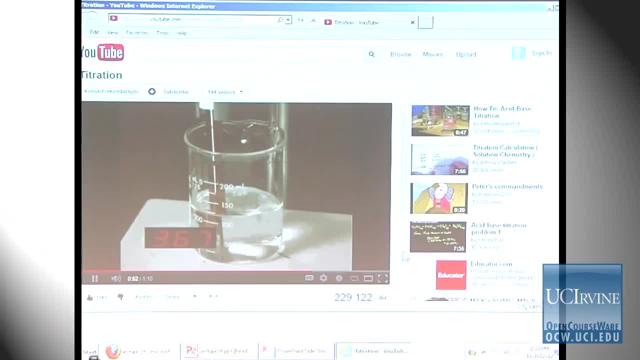 Initially the pH changes very little as base is added. Suddenly the pH changes rapidly as the end point passes. The solution quickly becomes very basic and again the pH changes very little. The end point occurs at this level and the pH changes very little. 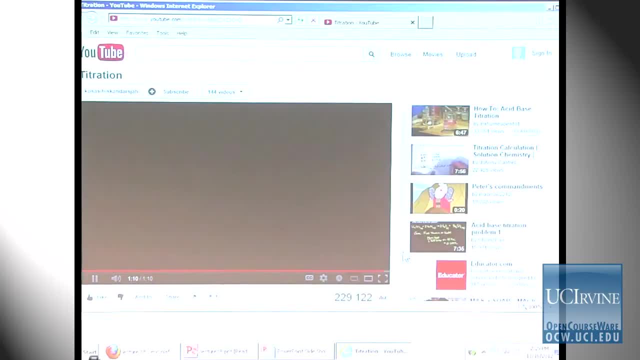 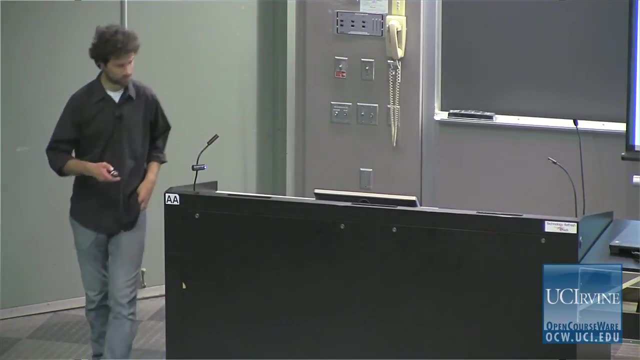 And the molecule: the end point is exactly at this point on the curve. The molecule: the end point is exactly at this point on the curve. Alright, So that is the reaction. Thank you, YouTube. Uh, let me tell you something about the pinkish color that you saw. 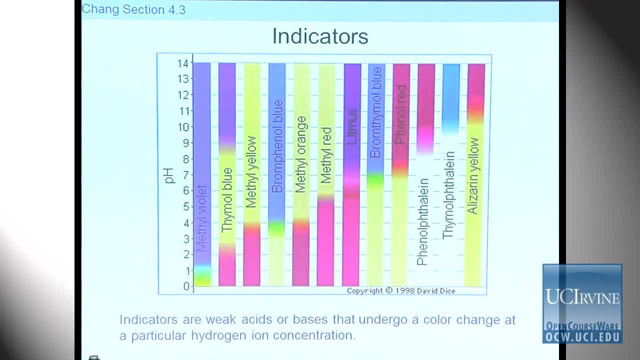 And uh, this is a this little, this little segment here I'm introducing is the cruise life long. It's not part of any exam, It's just extra information, just to give you an idea. These are, these things are called indicators. 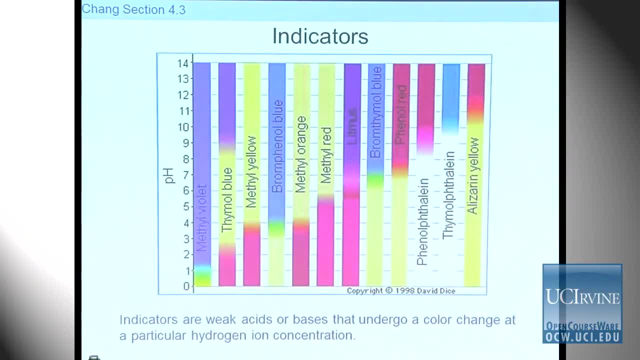 The way you use them is you don't have the average time, the average alpha, the average number of times you use that is, that is the average number of times you use the element that gives it a color are called indicators. These are just molecules that are floating extra in solution. 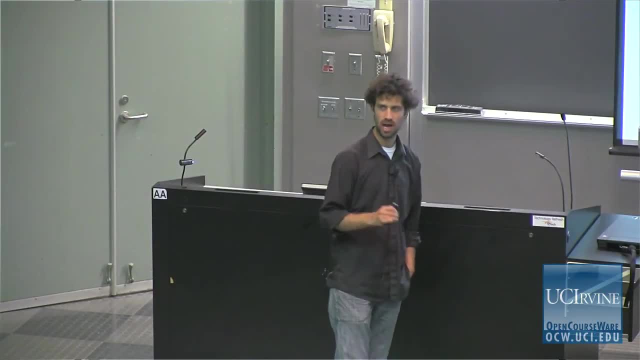 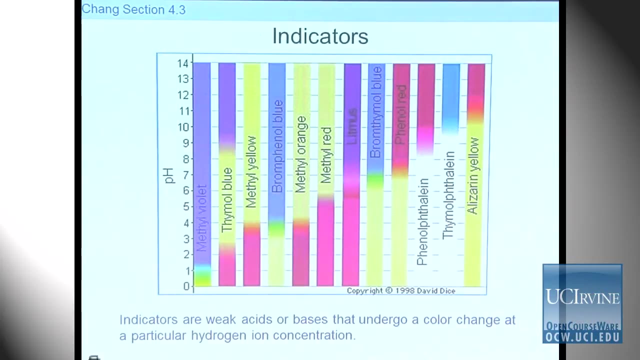 and these molecules can sense what the pH is, how many H plus ions there are. In other words, they assume a different color depending on the concentration of H plus ions in the solution. Now I'm going to give you an example of how that can work. Here's one. This is a phenolphthalein indicator. 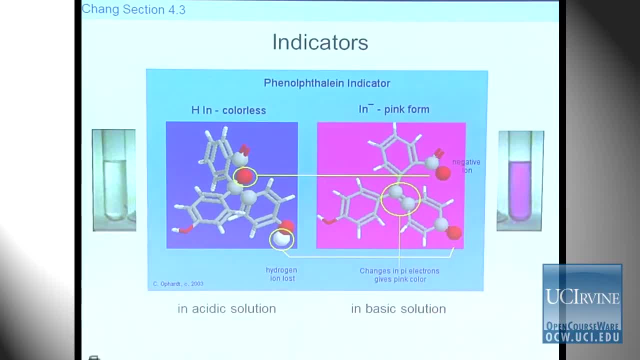 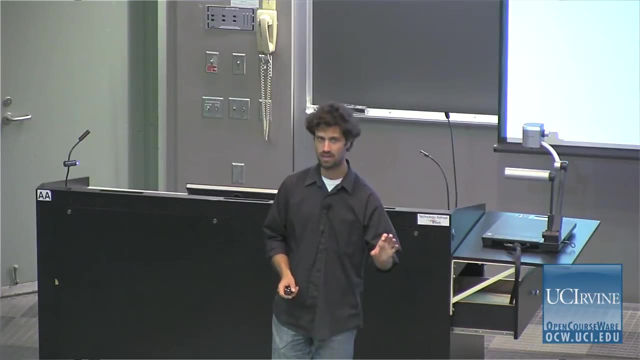 Here's the structure. it looks a little bit dramatic, but what happens is if the pH- the number of H plus- is very high, this part of the molecule will be so-called protonated. There will be an H plus sitting here Now, when the solution becomes more basic. that means there's a very high chance that this H plus will come off and not come back. 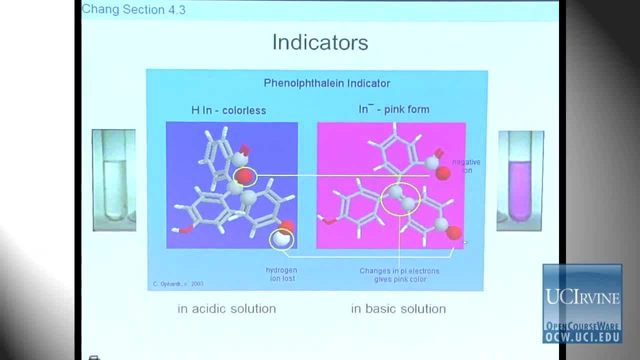 If that's the case, if H plus goes away, then this unit becomes different. this protonate, This double bond, clicks here, this one clicks there and forms a double bond in this location. That change in molecular conformation leads to the pink color of this molecule. So the molecule literally changes color because there is an H plus attached to it or not. 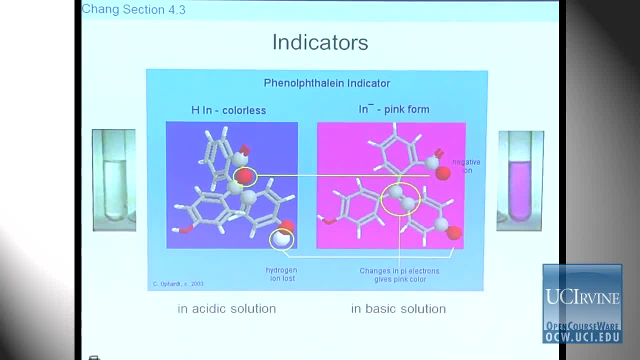 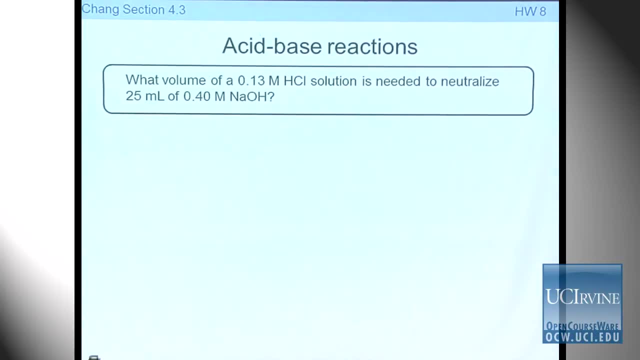 This is how molecules can tell you something about what's going on in solution, only in the molecular level. Let's do a little calculation with this kind of neutralization reaction. So let's say I have, just like the movie, you have NaOH sodium hydroxide in a beaker, okay, 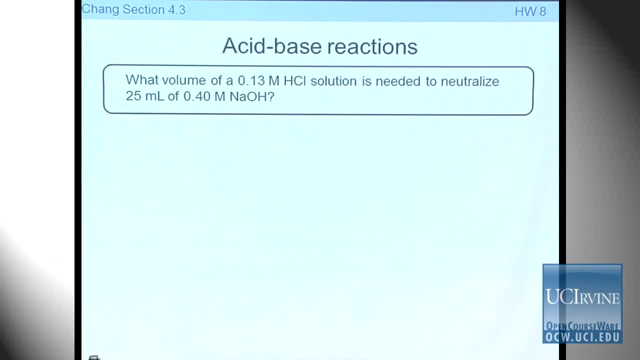 and you have 25 milliliters of that stuff and the molarity is 0.4.. and then I want to neutralize the solution with an HCl solution, and then I want to neutralize the solution with an HCl solution. 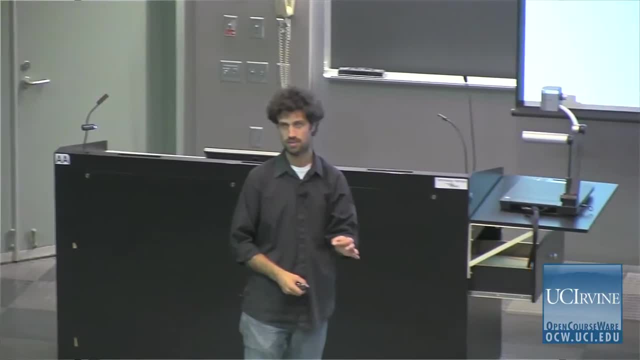 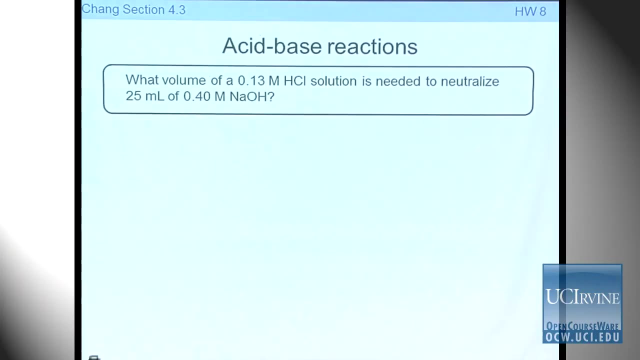 and then I want to neutralize the solution with an HCl solution. I have HCl in my量 and I'm going to add some of this. the concentration is given to till it is neutralized. The question is: how much do you have to add? What is the volume of this neutralizing acid? to neutralize only OH-λ. 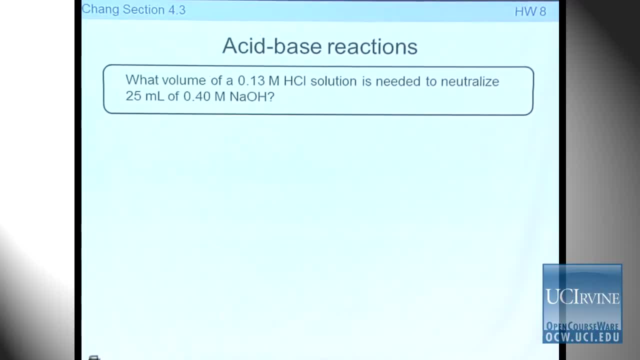 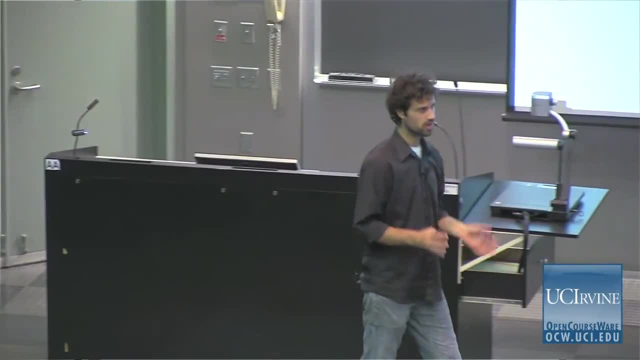 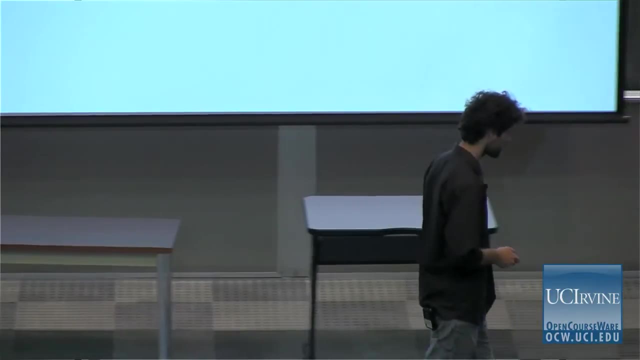 to neutralize only OH-λ. Okay, so let's do this. As always, we'd like to understand what is the system, we are talking about, what is going on. So one thing you can do is just see what kind of ions are in that solution. I have evidently H+, I have Cl, I have sodium and I have hydroxide. 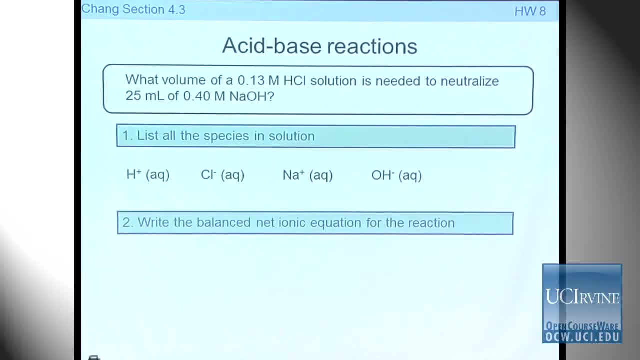 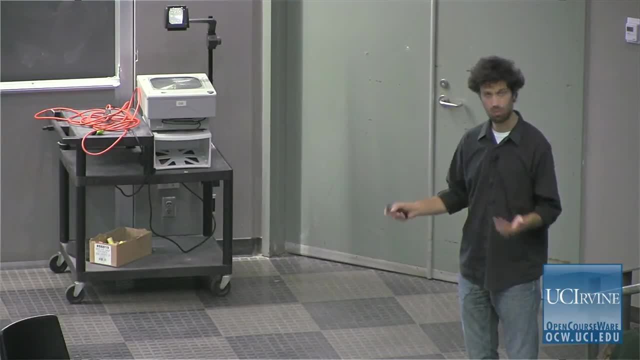 Then I'd like to find out what are the actual reactions taking place here. So this is the reaction you've already seen in several forms. This is the H+ reacting with the allyl kinase to form water. So this is the net ionic equation. 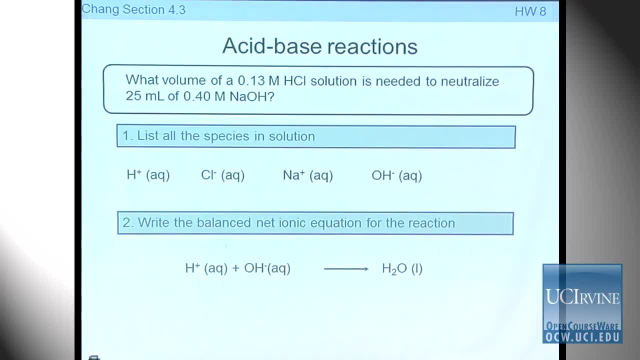 Cl and Na are just liquid ions. H+, one H+, one part of H+ or one mole of H+ reacts with one mole of OH- to form one mole of water: One-one-one ie mole ratios. Now, previously, the next step would be to determine: 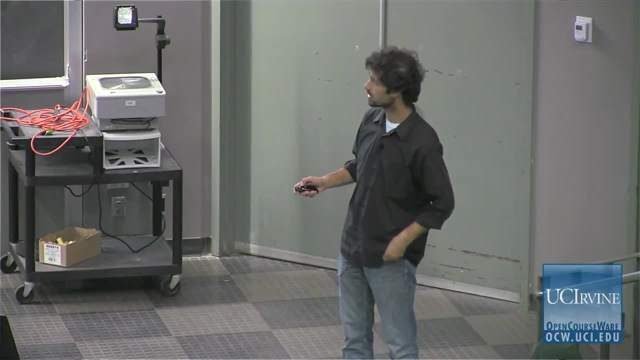 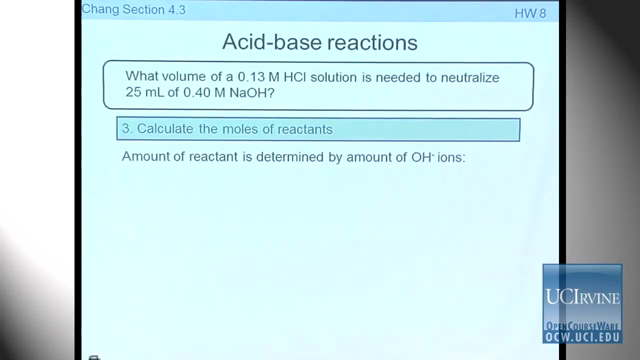 which one of these guys is the limiting reagent? which one of the reactants? I have two reactants: H+ and one H+. Which one is the limiting reagent? In this particular case, you probably don't have to do that. 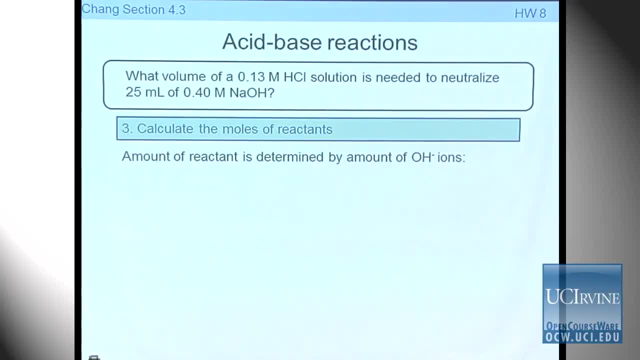 Because the question says you just have to add enough H+ to neutralize all the OH-. So that basically means that the OH- is the limiting reagent. You just have to add enough H+ so I have the same amount as the OH-. 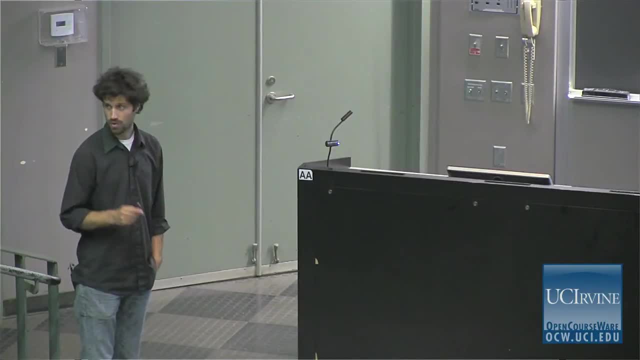 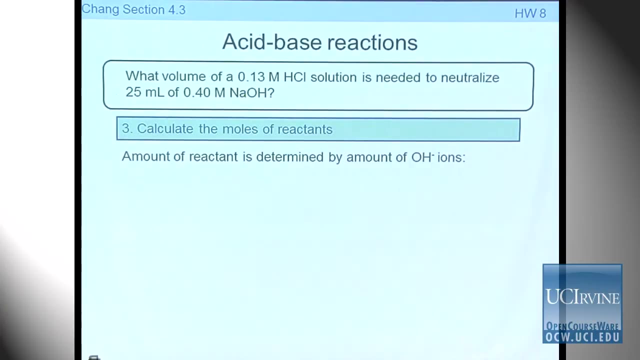 I'd like to know the number of moles of OH-, The number of moles of OH- that I have, The number of moles of OH- that I need to neutralize. So how do I do that? Well, I have a volume and I have a molarity. 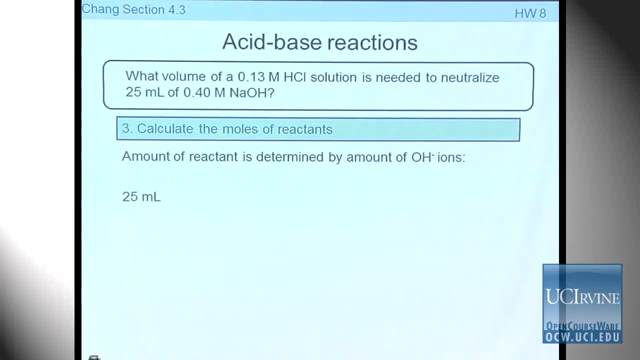 So I take the volume and V times M equals the number of moles. But this is in milliliters and molarity is in moles per liter. So I convert this very quickly into liters. 100 milliliters in one liter ml strikes out. now this is in liters And then multiply it with the molarity. 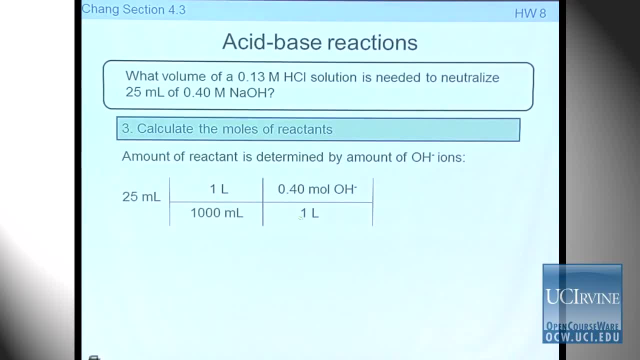 Okay, 100 milliliters in one liter. ml strikes out- now this is in liters- And then multiply it with the molarity 0.4, 0.4 moles per liter. If I do that operation, I have the number of moles. 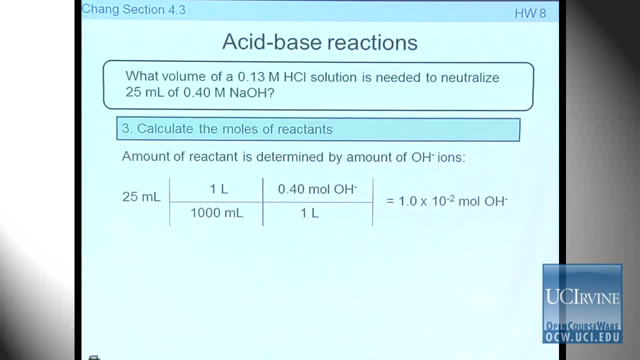 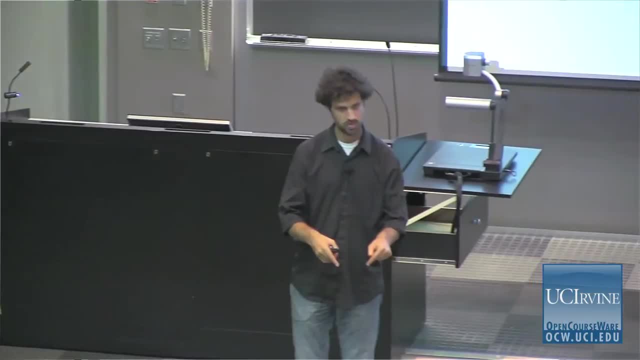 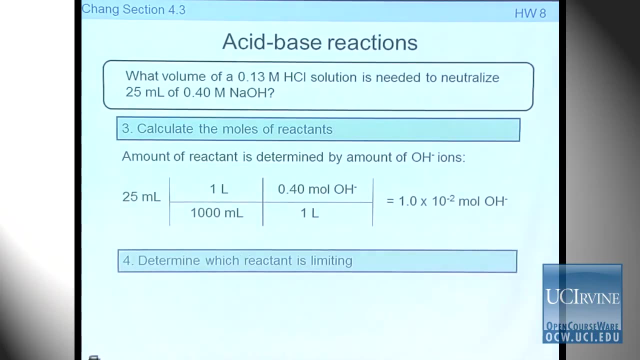 And it turns out to be a nice number: 1.0x10-2 mol OH-. This is the amount of OH- that I have in my theater. So now I know the number of OH- in my theater. Okay, I said already that there's not gonna be a limiting reagent on the H+ Right. put every image color on the chart. So point 4, 0.4 moles per liter, You're gonna do the operation. I have a number of moles in OH- And it turns out to be a nice number: 1.0 times 10-2 moles per H31.. 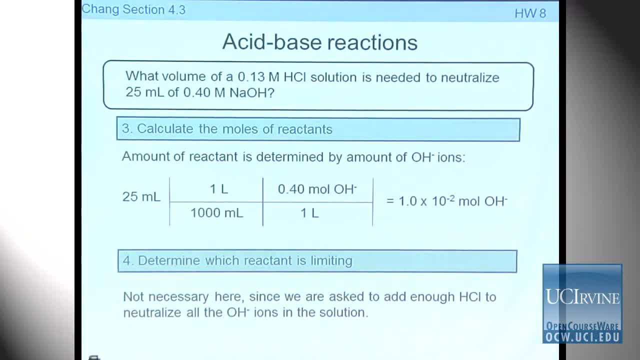 0.510 cons. 1.10, 0.2 Moles per Molic Ha soldant days from the middle ages to the middle ages, a limiting reagent. here I just have to add enough H plus to neutralize all these guys. 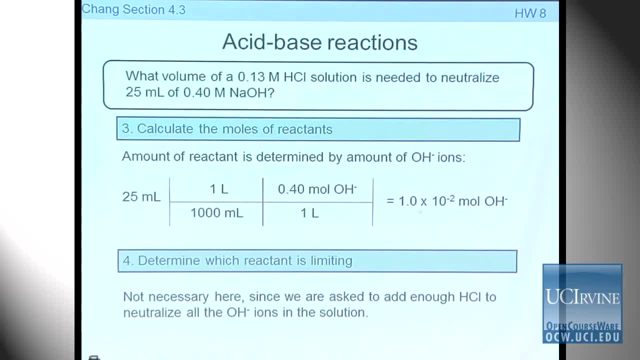 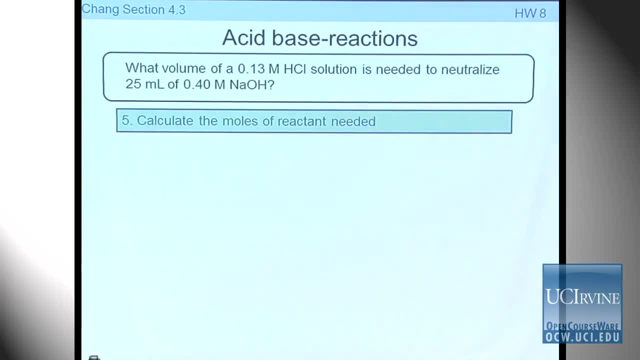 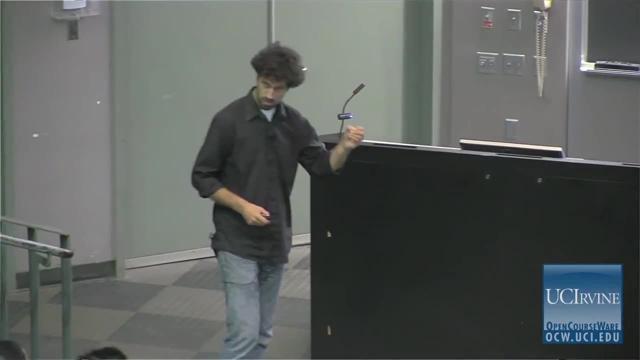 So I have to know how many H pluses do I need to neutralize 1.0 times 10 to the minus 2 moles of OH minus. I need to know the mole ratio between the two. So for 1.0 times 10 to the minus 2 moles of OH minus I need: 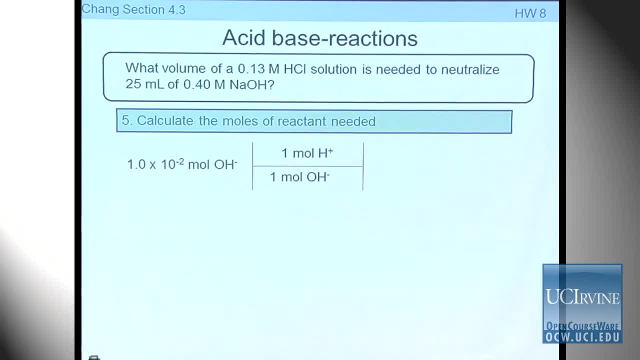 to multiply by the mole ratio of how these two things react. So for each 1 mole of OH minus I need 1 mole of H plus. In other words, I need just the same amount of H pluses that I have, as I have OH minuses in my meter. 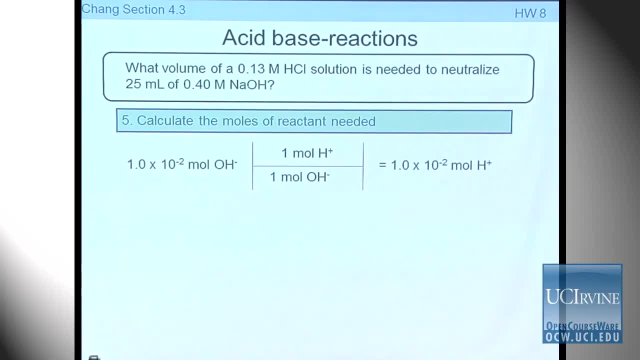 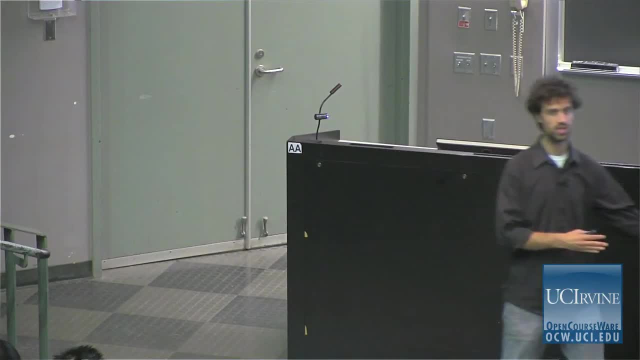 1.0 times 10 to the minus 2 moles of H plus. You can do this directly, right? I mean, if know that they react one-to-one, you can immediately say: okay, if this is how many moles of OH I have, that's exactly how many moles of H plus I need to neutralize it. 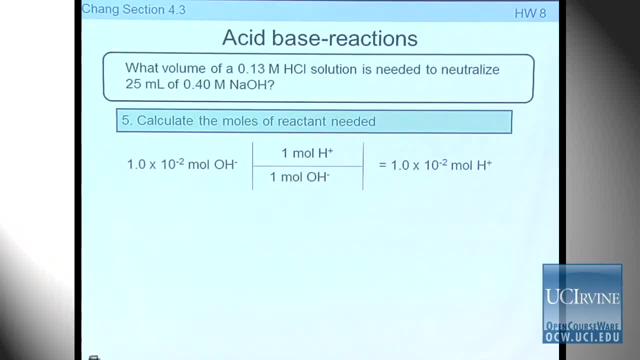 but I'm sure you can always use these mole ratios, which are always right and always guiding in the right direction. So this is the number of moles. I need to know the volume. How do I do that? Well, I have the number of moles. 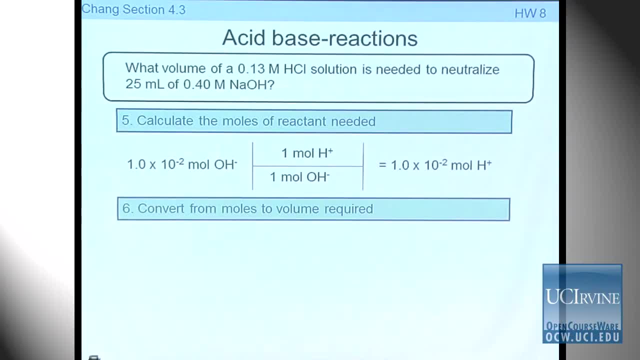 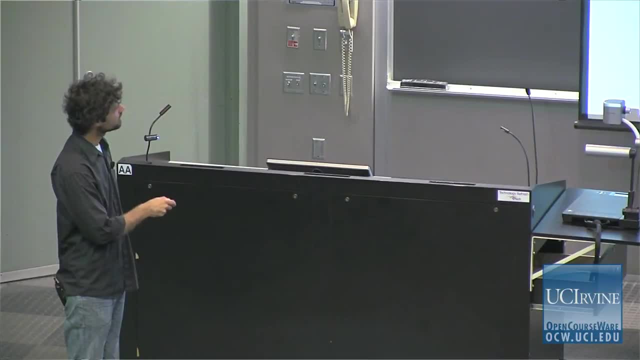 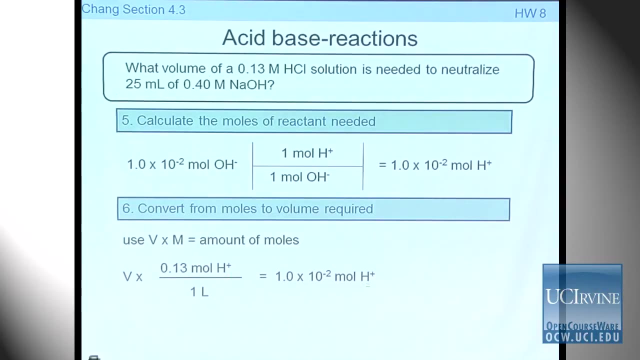 I have the molarity and the only missing parameter is the volume. So I know that v times m equals the amount of moles. I have the amount of moles, I have the molarity and v is equally unknown. Okay, So these two values are given. this is the molarity of the solution. 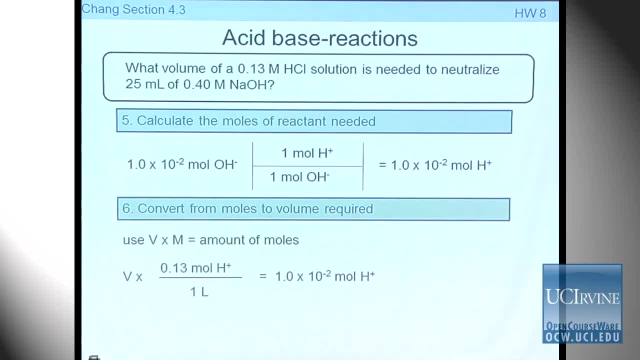 that is the amount of moles that I need. so if I rearrange this, I find the volume of the solution that contains this many moles of H+, And that is this number divided by this number: 1.0 times 0.2 moles divided by: 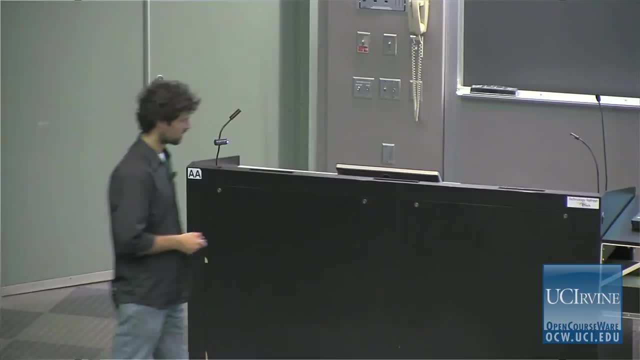 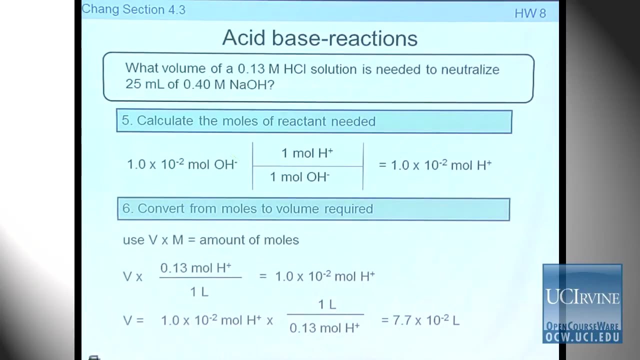 0.13 molarity and that equals 7.7 times 10 to the minus 2 liters. This is the volume that contains this many protons to neutralize this many mole H-maxes. Okay, One more question. Yes. 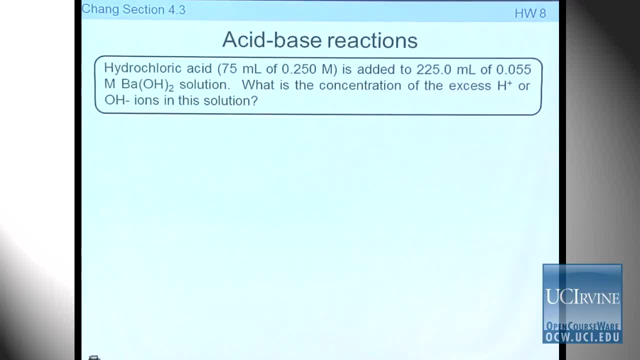 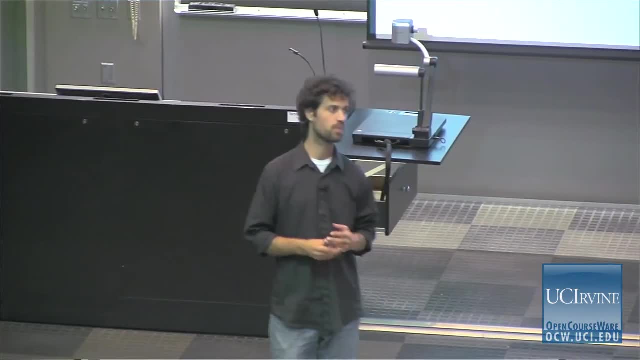 One more question: Instead of doing all the six steps, we can just do m1 and then b1 and then 2 times b2 and then just start from here. Okay, I see that from this angle, And then I'll just go from there. 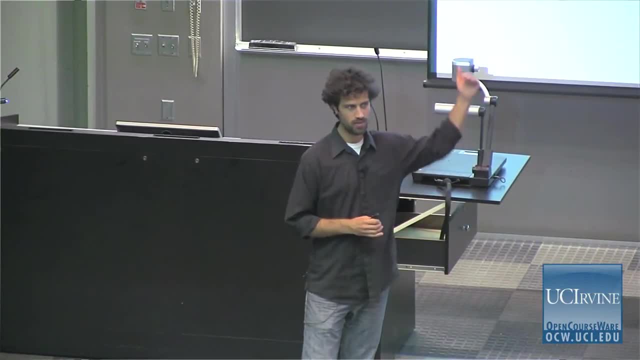 I know we're not going to be able to use this formula, but But even if you use this formula, I think what you can do is that you can at some stage- but you have to be careful when you apply that formula. This way, you actually approach the problem from understanding of what you're doing, rather. 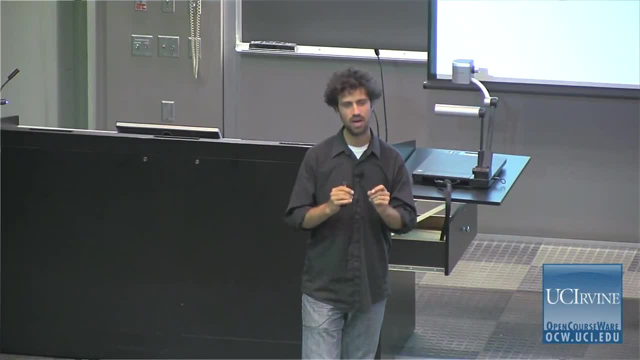 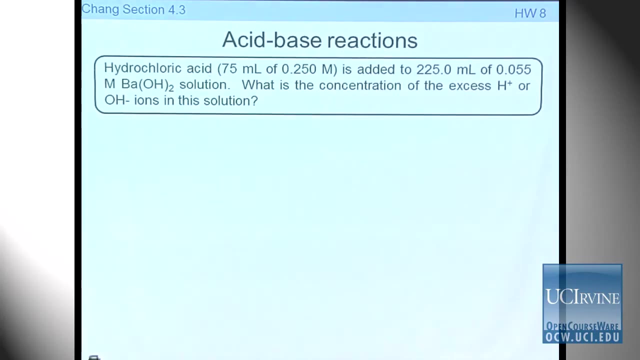 than blindly applying a formula and hoping you get it to a rat. You want to understand the problem and, based on your understanding, use the right formula. Okay, Okay. Another example: hydrochloric acid is added to barium hydroxide. 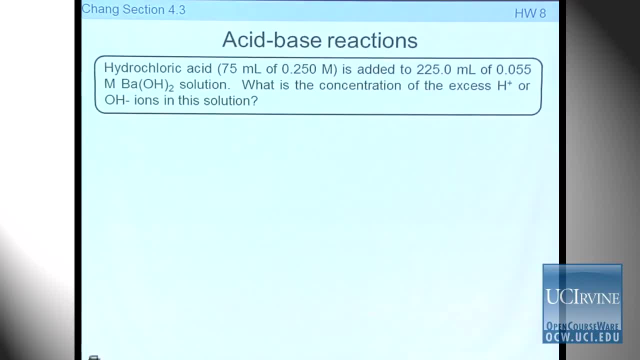 and, luckily for me, the volumes those are in consumes: 1.1 and 2%, right, Okay, younger level with this ea normalization of nano tales, warp and the molarities are given for each solution and that means I can immediately get to the number of moles in these things. 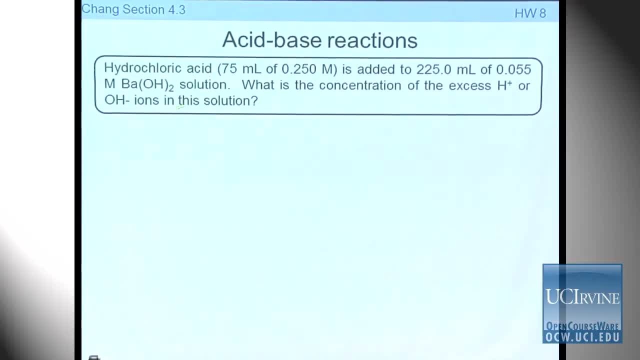 The question is: what is the concentration of the excess H+ or OH- high-agent solution? So I throw these two things together. clearly this is an acid, hydrochloric acid. clearly barium hydroxide is a base. I throw them together, a reaction happens. 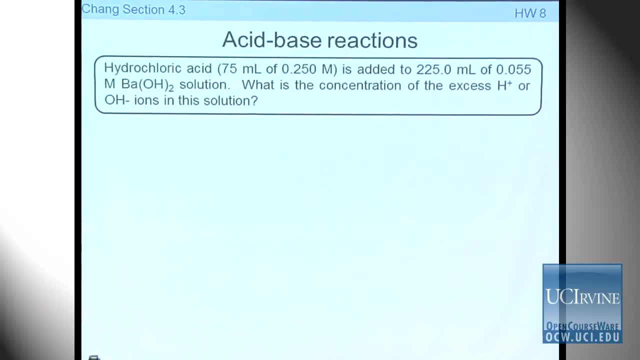 an acid-base reaction happens, the H+ and the OH- react for water and then, when the reaction is done, either there is H plus left or OH- left. That's what I have to determine, Determine which one is left and how much of it is left after the reaction has come to a stop. 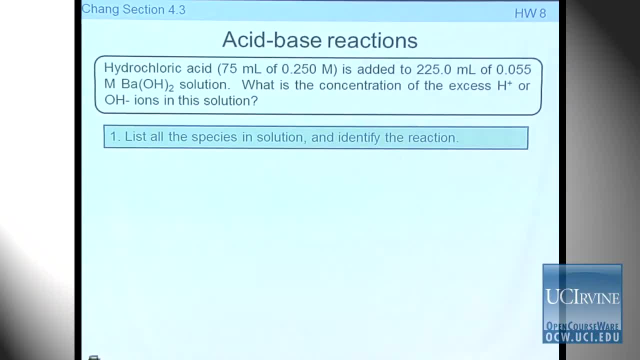 So again, I'm starting from the very beginning. I just want to see what am I talking about. here are the ions in solution: H+, CO-, barium 2+ and OH-, and the reaction that has taken place is again the same. 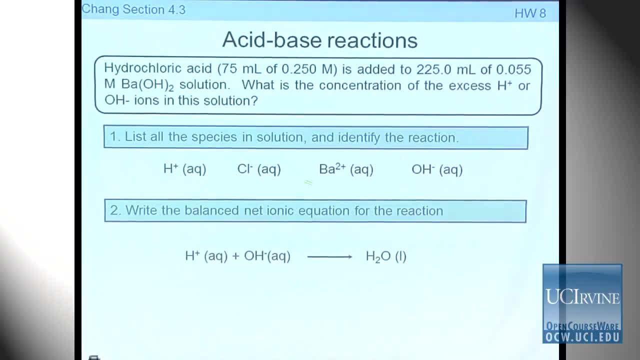 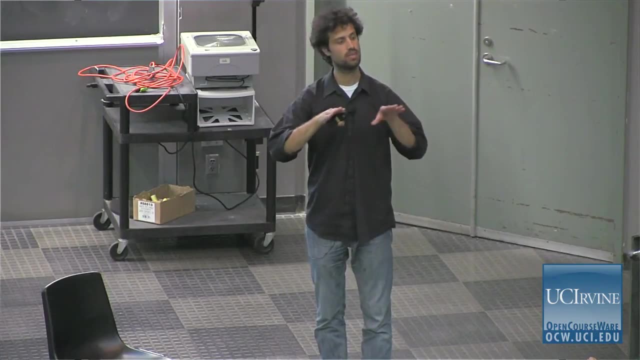 H+ and OH- are for water, Cl- and barium are just spectator ions, Okay. so what I really want to know, then, is: how many H pluses do I have, how many OH- do I have, and which one of these is the limiting reagent? Which one is running out first? 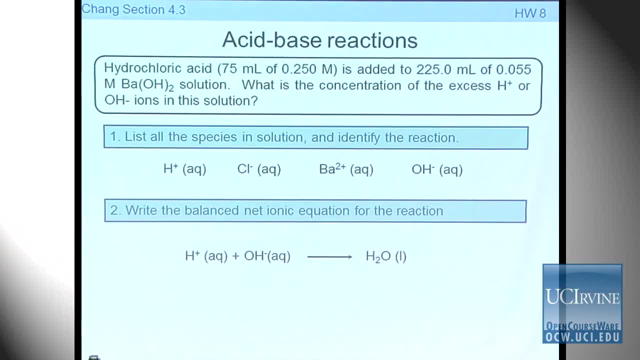 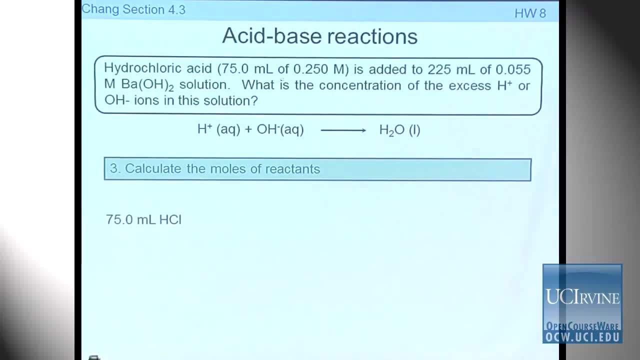 Okay, what other information should be- obtainable from the information here? so here it is. I'm looking at and calculating how many H pluses I have from the amount of dish hyaluronic acid that I have Sleep. this is the volume. 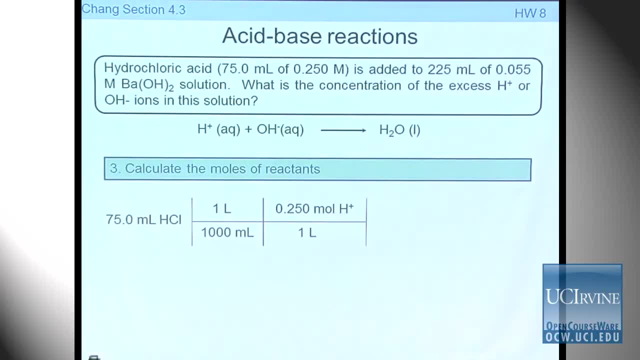 I've converted the volume to liters and then multiplied that by the molarity of HCl. A mighty of HCl is 0.25.. I also see immediately that each HCl molecule has 1 H+. Okay, So that means if you do this operation for HCl you have the same amount of H pluses as you have HCl molecules. 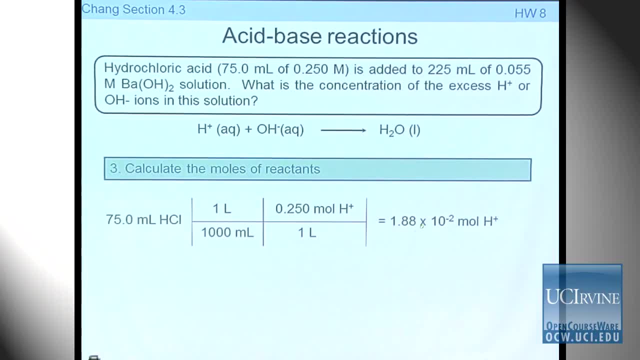 So what I have after this operation is 1.88 times 10 to the minus 2 moles of HCl, and that's the same as the number of moles of H plus, Because each HCl only has one H plus. 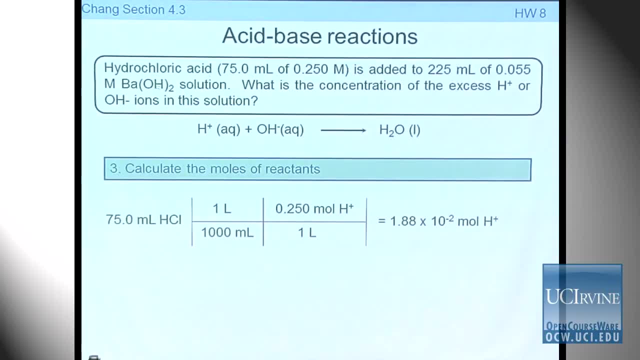 Number of moles of H plus number of moles of O I also need. so let's do that. This is the volume of the barium hydroxide solution. It's already in liters, So I just multiply that by the molarity of the solution. 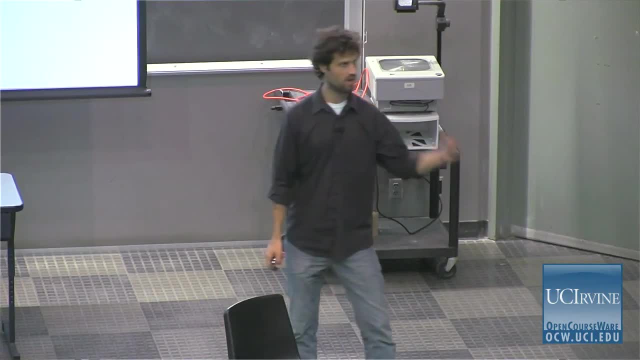 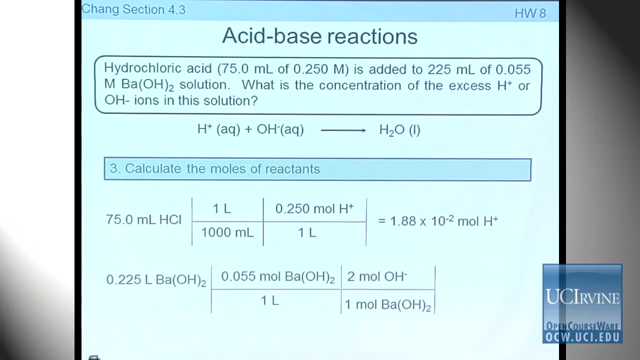 And if I do that, I get here the number of moles of barium hydroxide units, But each unit has two OH-minuses. so I have to do the following conversion: Convert from the unit of barium hydroxide to the number of OH-minuses. 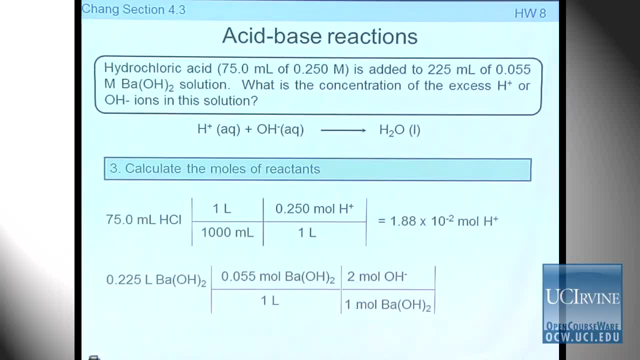 Here I had 1 to 1. Here I have 2 to 1. Each 1 mole of barium hydroxide produces 2 moles of OH- because of the substrate 2 here. So that gives me 2.48 times 10 to the minus 2 moles of hydroxide NaS in solution. 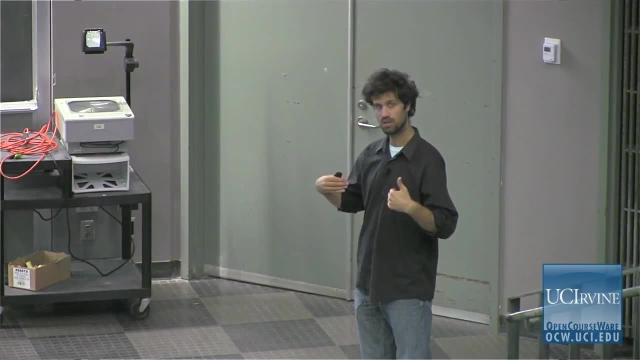 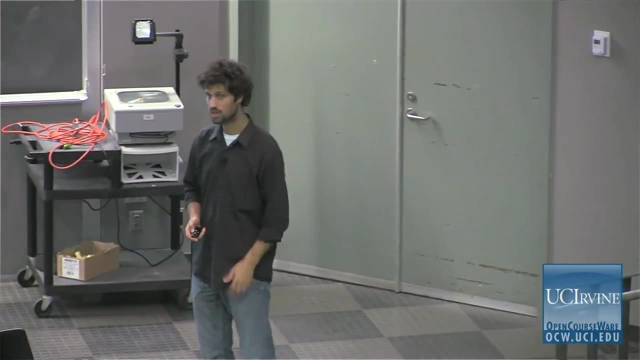 Okay, That's good. Next step for me is to determine how these things react. what is the mole ratio and which one is the limiting reagent. You can do this very quick or you can do it efficiently. The quick way to do it is: 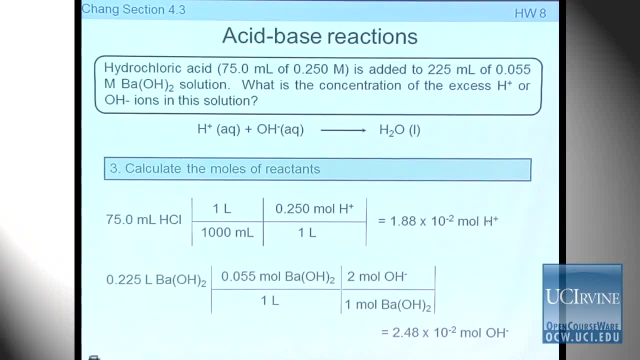 I know they react 1 to 1, H plus or H minus. I have less of H plus and more of OH minus. so if H plus runs out first, H plus must be the limiting reagent. But if you do it the official way, you should find the same thing. 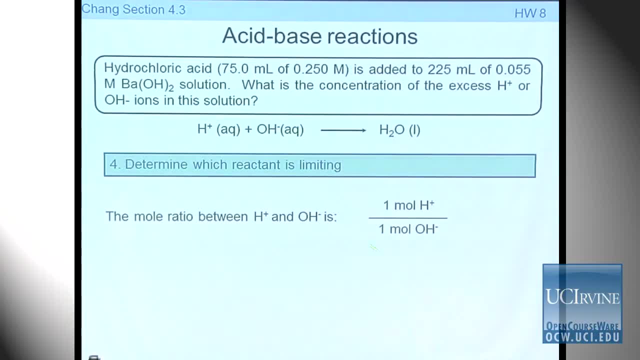 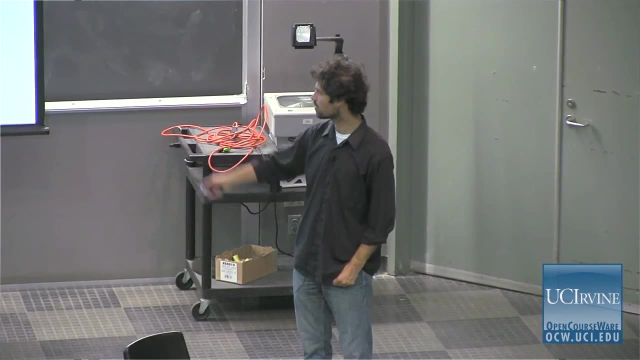 So let's just double check. The mole ratio, according to the equation here, is 1 to 1.. So the ratio is 1. And the ratio that I've calculated from the actual amounts of the compounds is 1.8 divided by 2.48,. I've just calculated these numbers and that is less than 1, meaning the numerator is the limiting reagent. 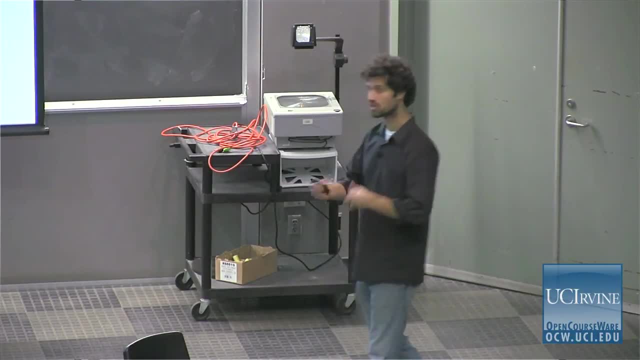 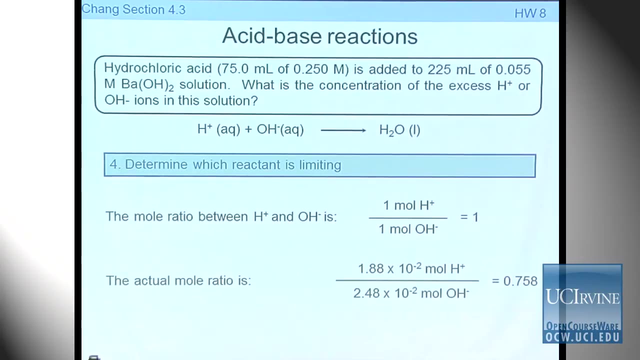 That's exactly what I found. So you can always double check whether your intuition is correct. So I take the number of H pluses then and calculate how many OH minuses I have left, Because OH minus is the excess reagent. 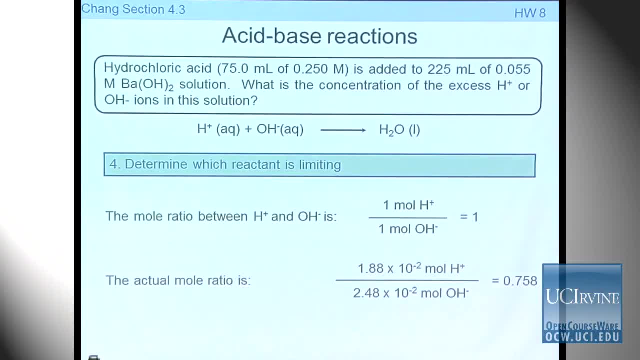 After the reaction all the H pluses are gone, But OH minus is left, because OH minus is in excess. So the question then is- the first part is this: one is the limiting reagent. so I only have OH minuses left in the solution. 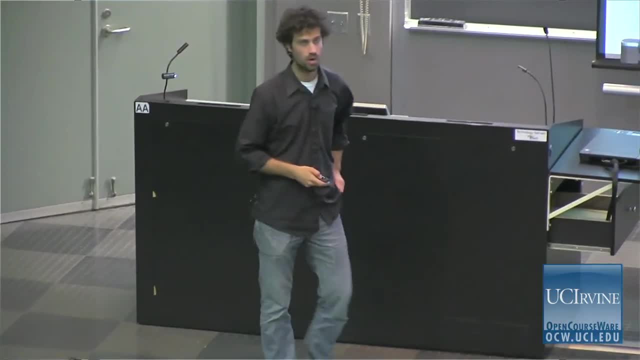 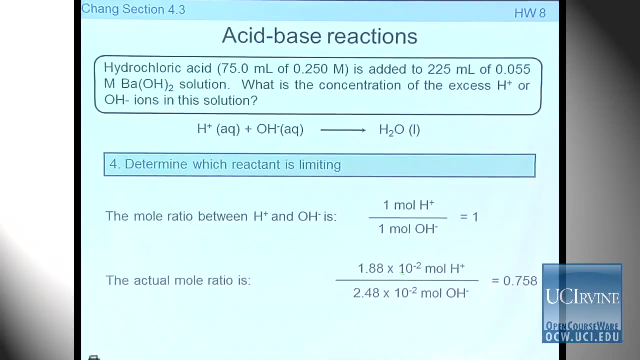 How many do I have left? Okay, The first thing I have to know is how many have reacted. Well, I know that they react 1 to 1 with H plus. This is the amount of H plus. That means this many of OH minuses will react. 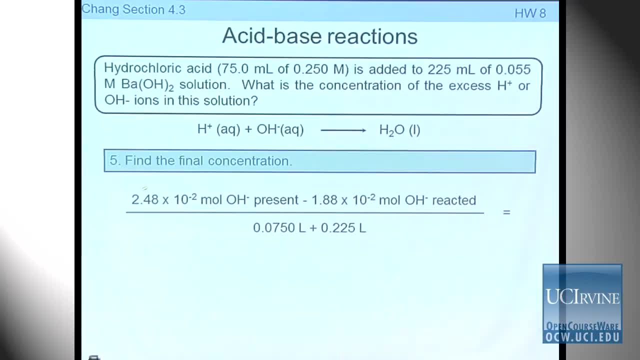 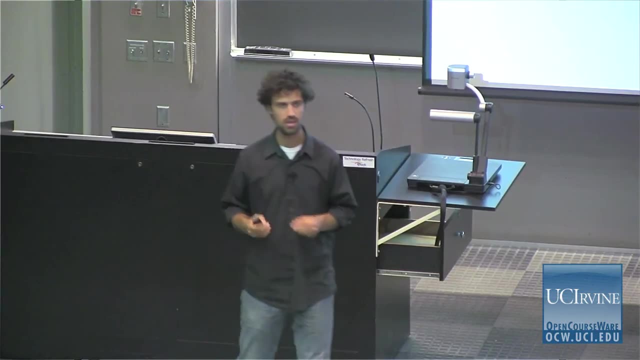 Okay, So this is what I had in solution previously at the beginning: 2.48 times 10 to the minus 2 moles. that is the total I started with, 1.88 times 10 to the minus 2 moles reacted with H plus. 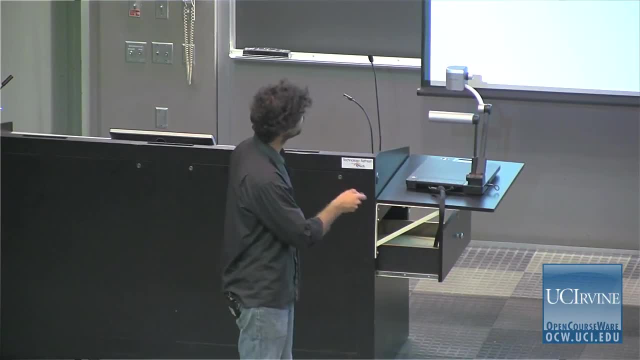 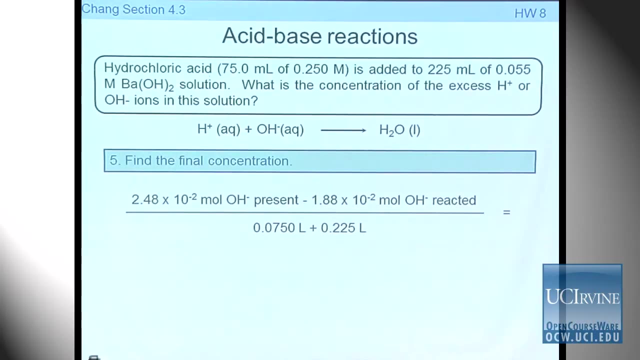 in a 1 to 1 ratio. So if I subtract these two from one another, I have what I left in the solution in terms of moles This times, that is, the number of moles of OH minus left after the reaction. Okay, 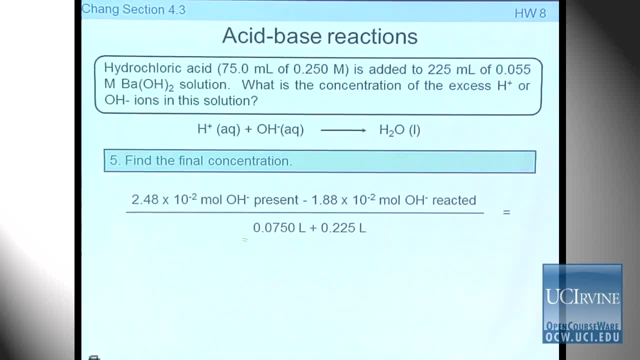 This is the number of moles of OH minus. This is the total volume. This volume plus that volume is here and if you divide the number of moles of OH minus by the total volume, you find the molarity of OH minus. 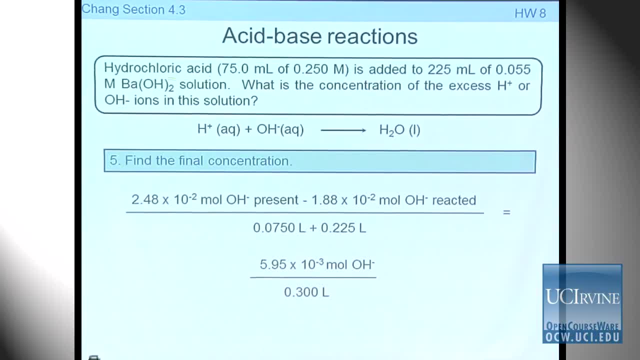 Okay, That's the real question here. What is the concentration of the excess reagent after the reaction? Okay, That's what I calculated right here. This is the total number of moles, That is the total volume of the solution. The concentration, therefore, is, in this case, 1.8..